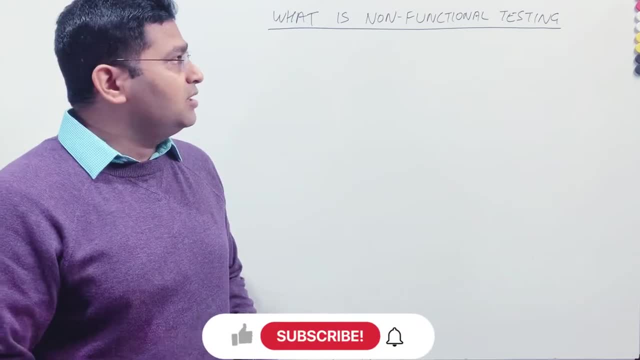 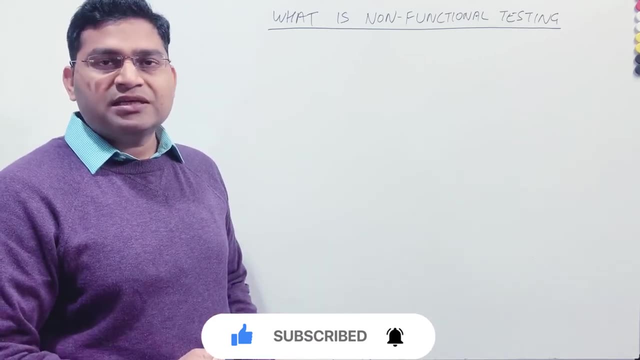 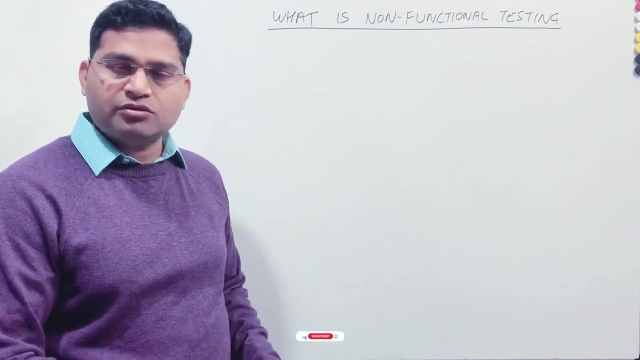 explain those in the interviews. okay, So let's start the non-functional testing. Prior to that I'll cover briefly about the functional testing. So in the functional testing in the previous tutorial we have understood that functional testing is testing the functional aspects of the application or the software. 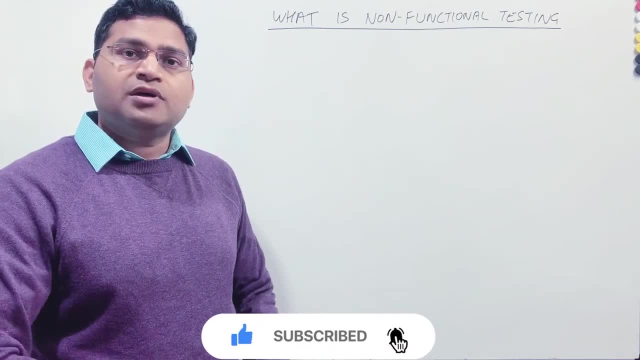 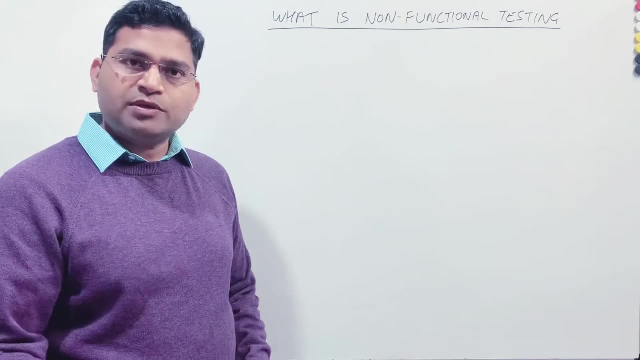 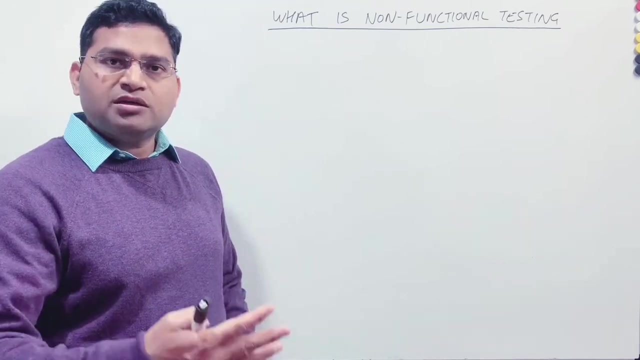 So what are the functional aspects? So functional aspects are the requirements that you get from the customer. okay, So I'll take an example of e-commerce website again. So e-commerce website is testing the feature or the requirement given by the customer to build that registration. 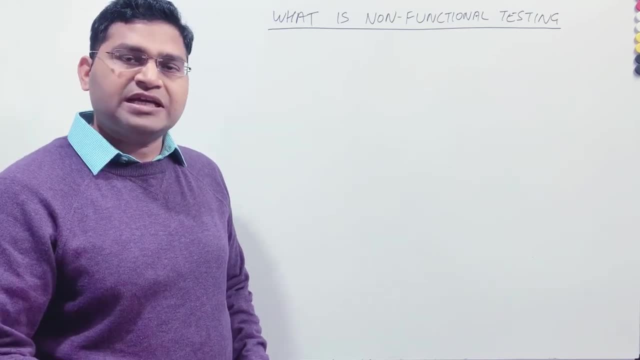 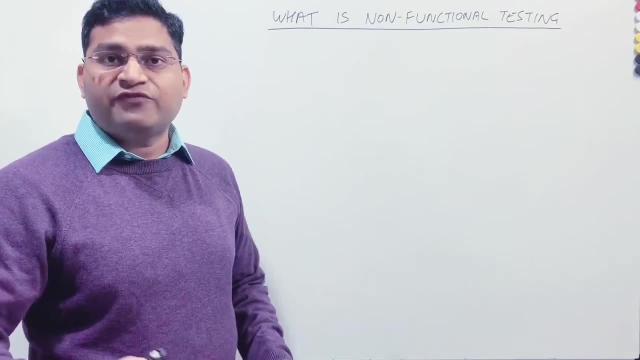 functionality. So when you are testing the registration functionality, you are trying to launch the registration form, provide the details and click on register link. That testing is the functional testing. Now, when we talk about the non-functional testing, non-functional testing. 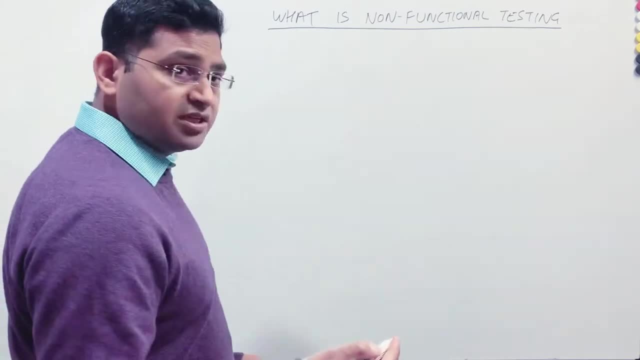 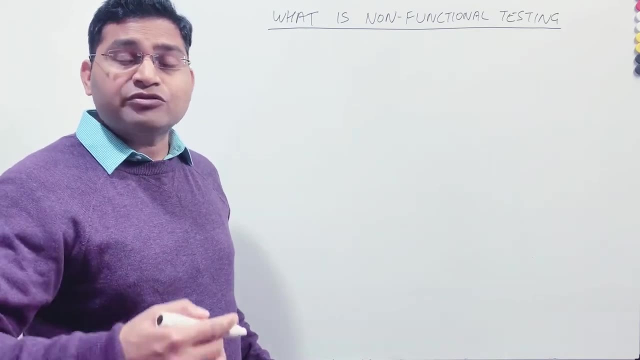 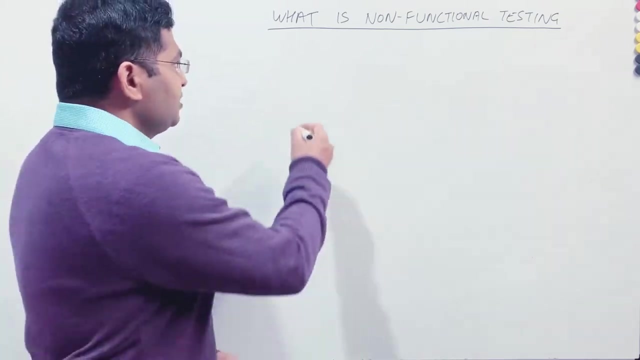 tests the responsiveness and stability of the application, right? So when you are testing about how the application is responding or how stable the application is, then you are testing the non-functional aspects of the application, right? So say, for example, this is the registration. 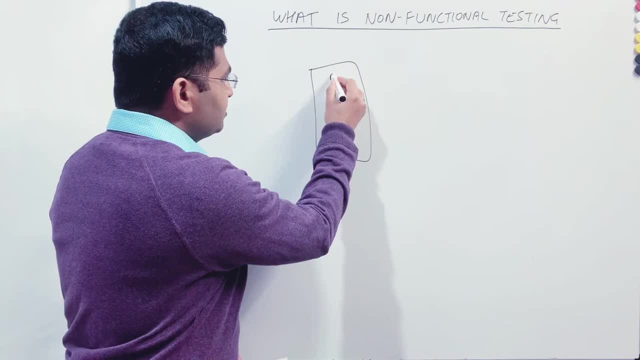 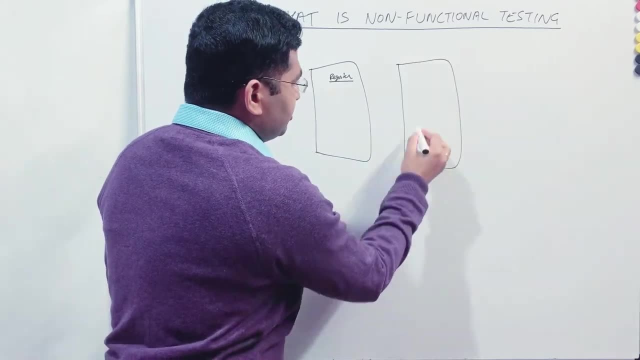 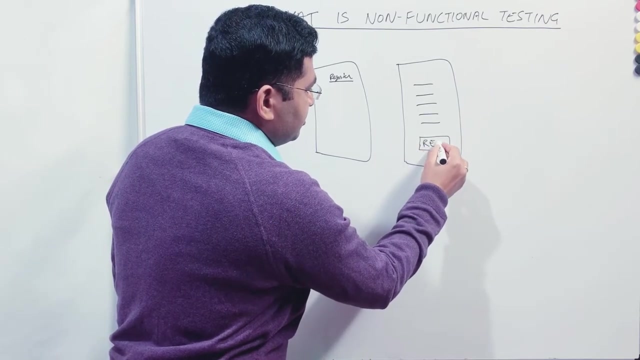 page, say, for example, of an e-commerce website, and this is the link, register link- right. When I click on register link, then it will open the register form wherein I have all the details of first name, last name, all the details, and then I have to click on register button And once I 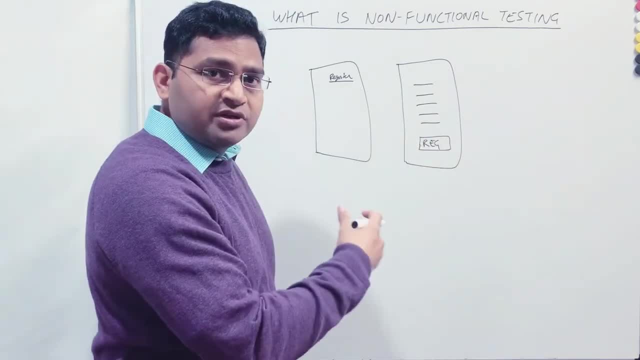 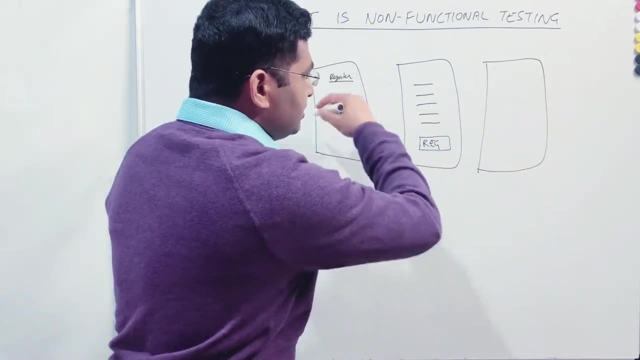 click on register link. then it will open the register form wherein I have all the details- register button, my user details. whatever details i have provided, i should be registered and should be redirected to the dashboard page. right, so this is something which is functional aspect. now, 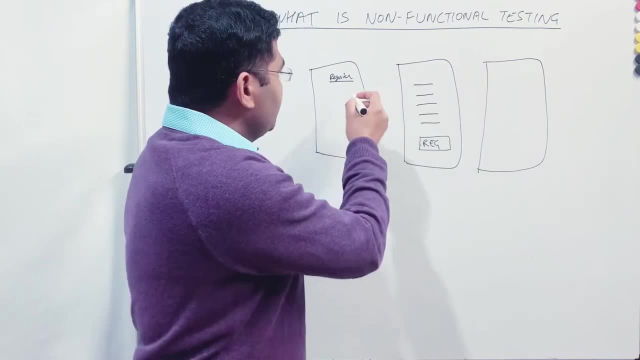 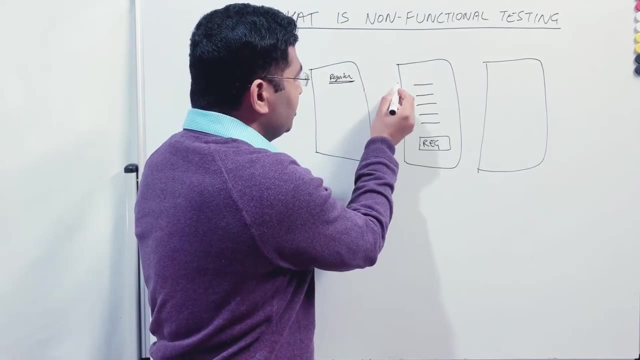 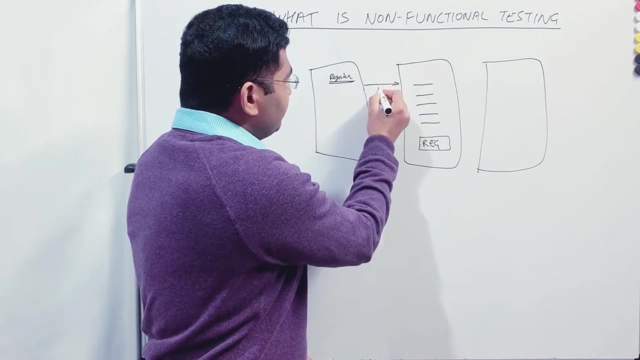 the non-functional aspect of the same operation would be, when i click on register button or register link, how much time or what is the response time to open the registration form? right? so if i am looking for this particular response time- say, for example, it is taking you. 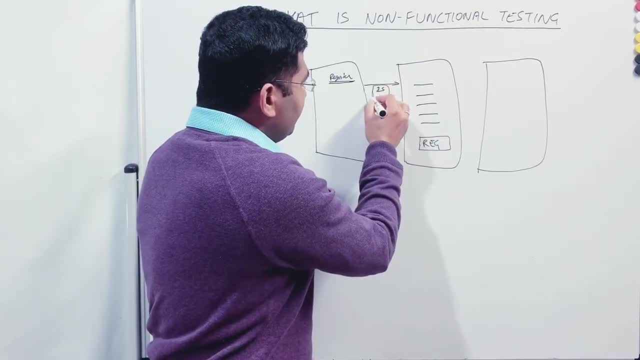 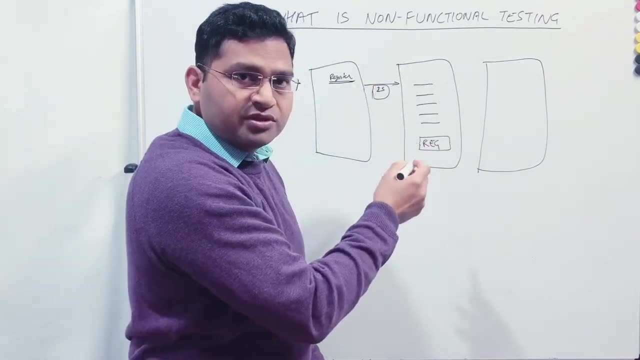 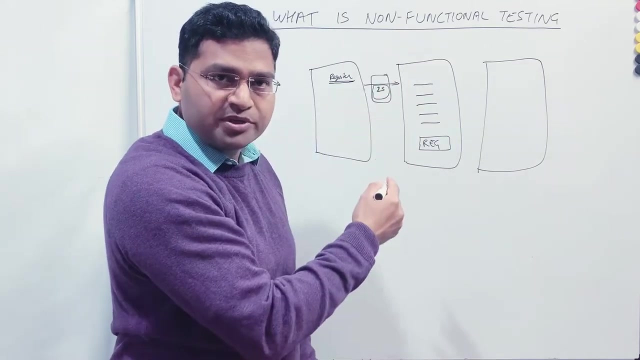 know two seconds, then if i am verifying this particular aspect- the response time- when i click on register link to open the register registration form, then this is known as non-functional testing. if i'm interested into the response time of particular operation, then that is non-functional aspect of the testing. similarly, once i click on register, 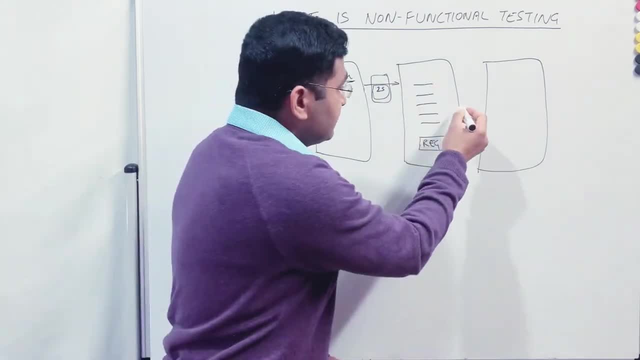 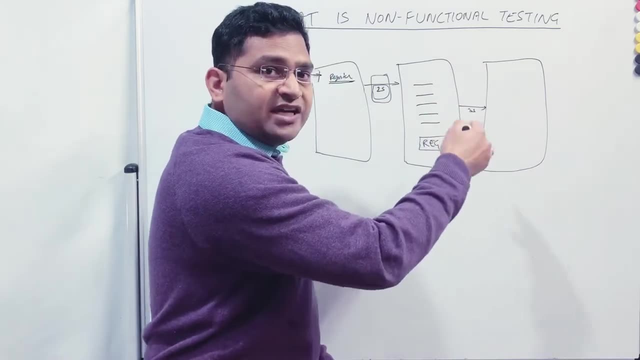 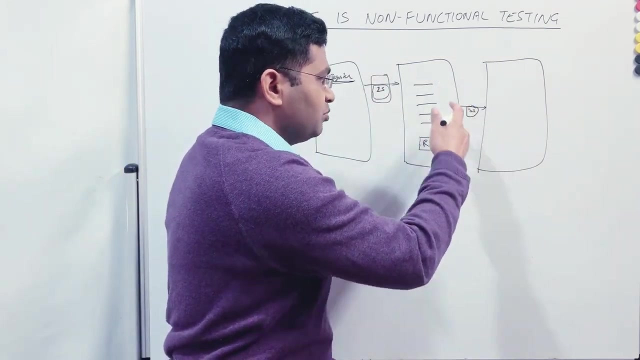 button here after filling out all the details, how much response time it took to basically redirect me to the dashboard page. so that is the response time i am verifying. so this type of testing that you do to verify the response, to verify how stable the application is, that is. 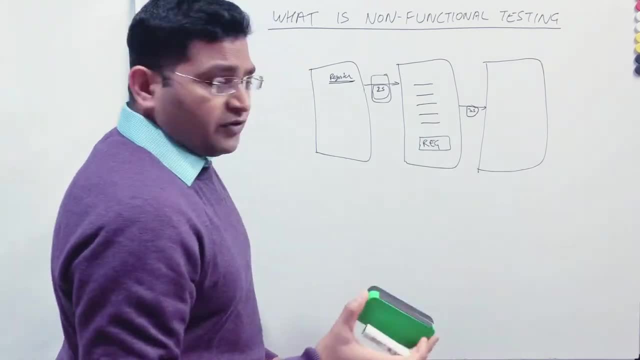 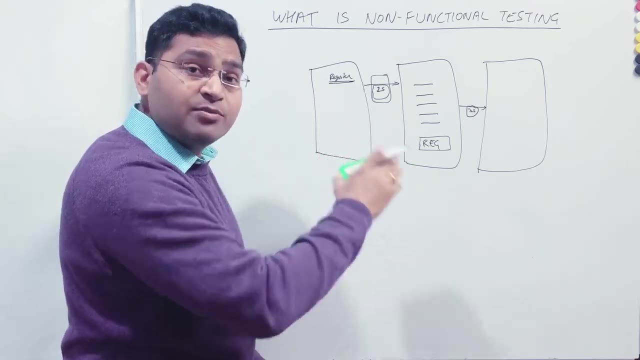 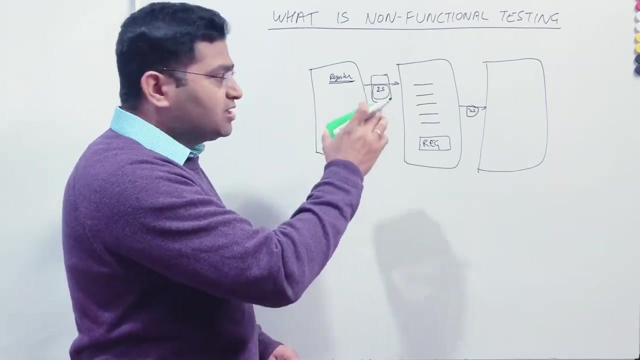 non-functional testing, right? so i'll cover this non-functional testing in a lot more detail, but this is brief. you know, introduction, what exactly non-functional aspect is the? there are many more non-functional aspect that you will be verifying in the non-functional testing, right. so responsiveness, or response time, is one factor of it. so that is um the brief now. 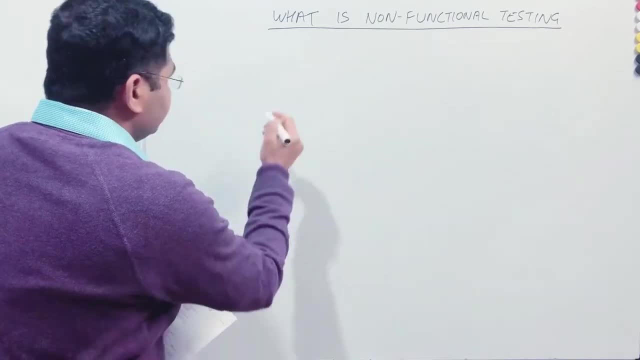 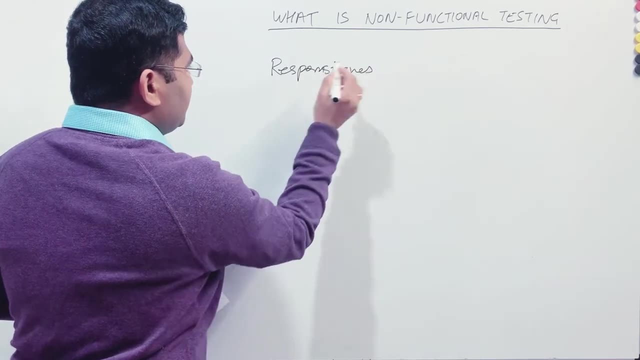 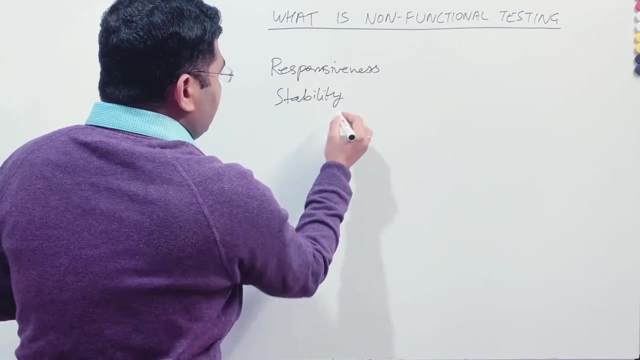 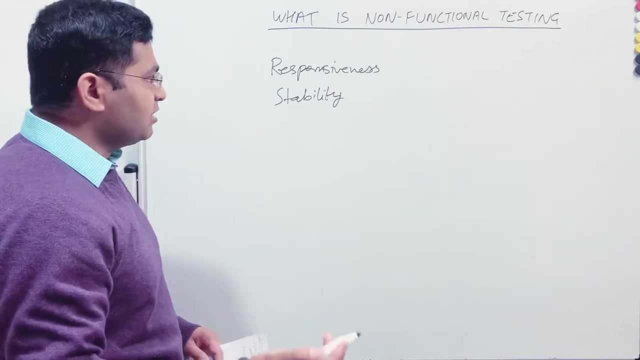 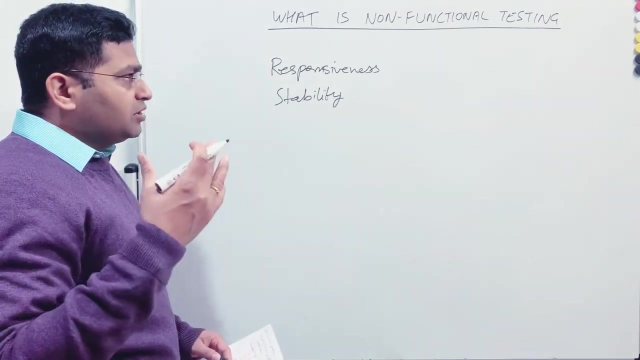 let me um. so the first thing we check is the responsiveness. so i'll write responsiveness of the application and then second, is the stability, right? so when we say responsiveness- how the application is responding on a particular condition- or the load- say, for example, in the festive season, e-commerce websites have lots and lots of load, right, so there will be a lot of people. 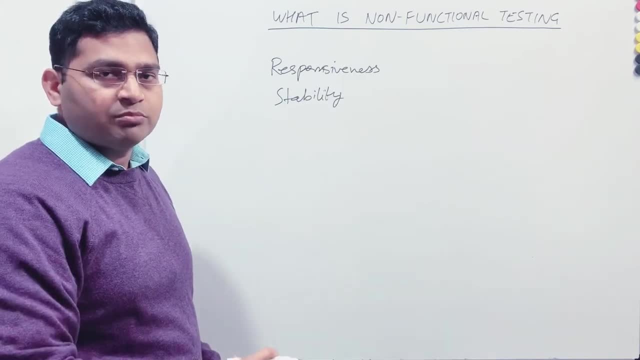 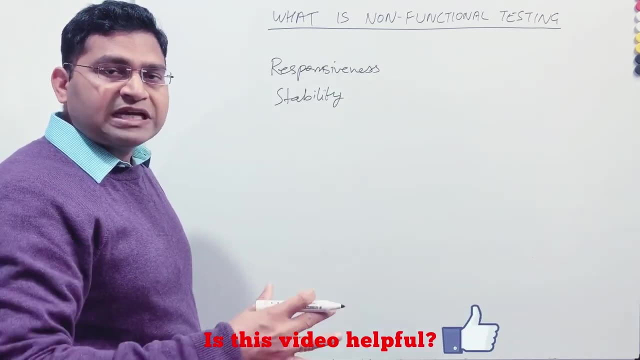 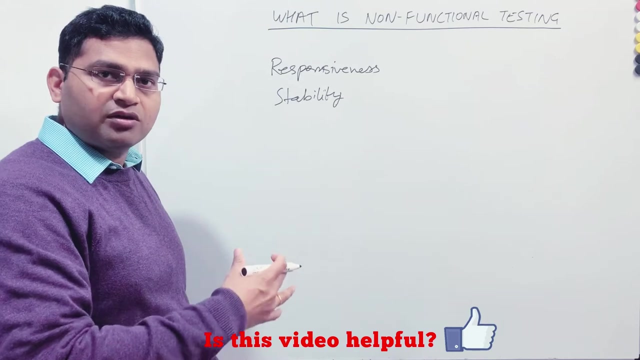 who will be buying the items from amazon, from ebay. so during the festive season there will be thousands and thousands of users, concurrent users, at one particular time to buy the item or say, for example, there is a sale declared or there is a sale on a particular you know day. then on that, 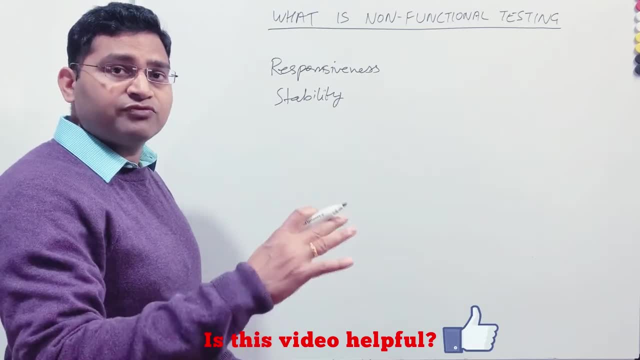 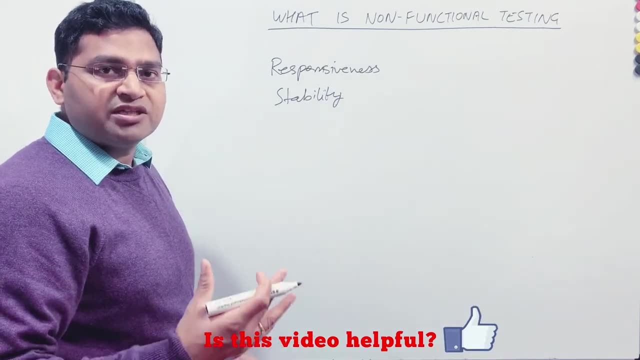 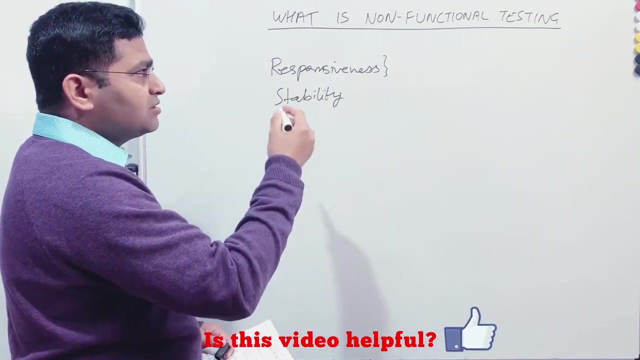 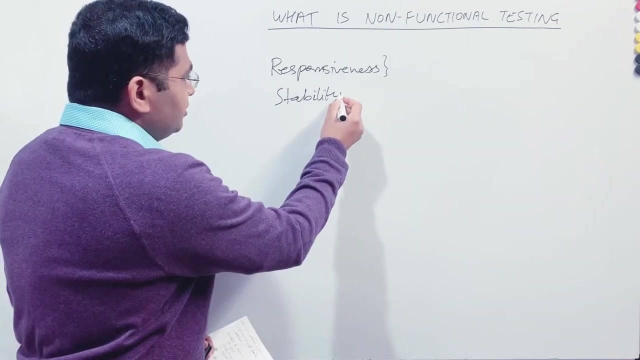 particular day there will be a huge amount of users or spike of users on the website and then in that particular condition, how the application is responding. so when you are verifying the responsiveness, then that is the non-functional aspect and that is non-functional testing whether your application is stable in those heavy load condition. if you are verifying the 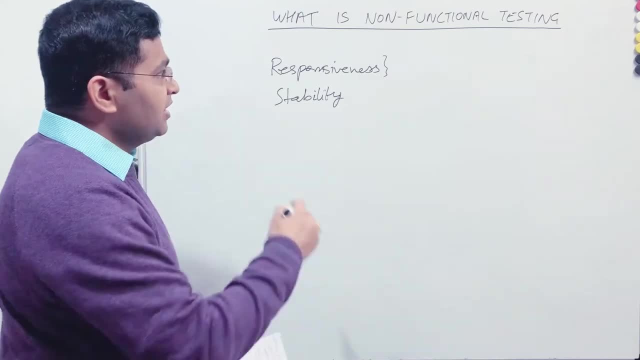 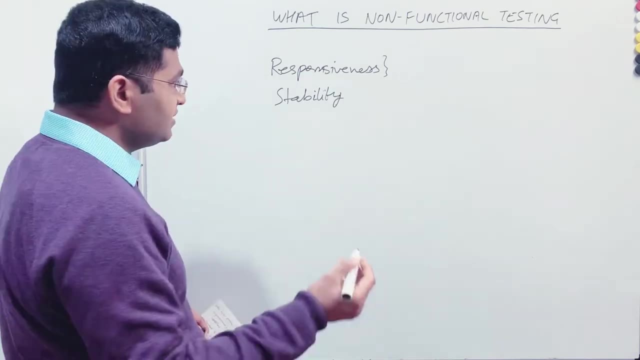 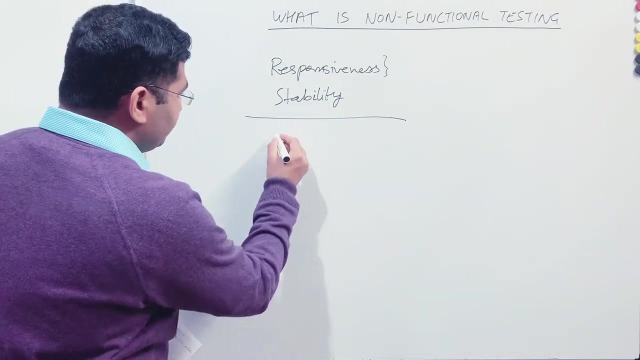 responsiveness and stability. this is non-functional testing. in the non-functional testing, what are some of the? you know, performance indicator basically. so when you do non-functional testing, you verify certain things. so there are many performance indicator, but i'll cover the the most common one. so the first one is basically the response time. right, so you verify the response. 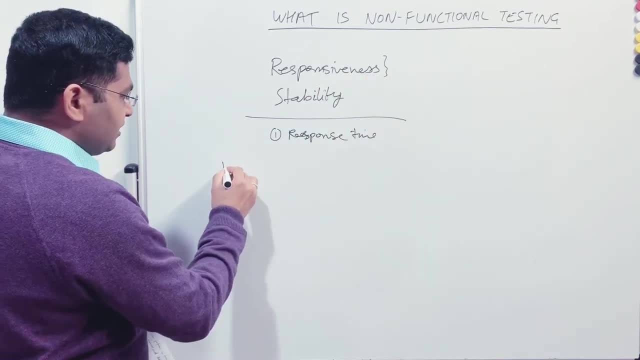 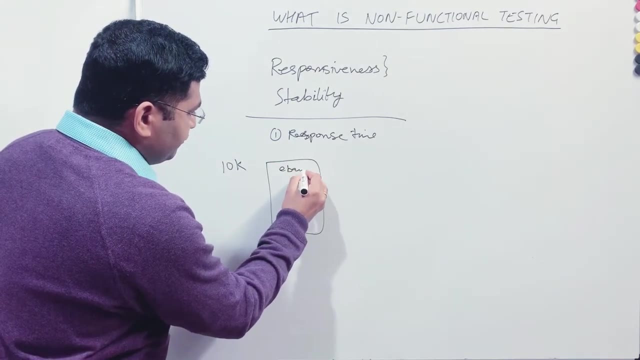 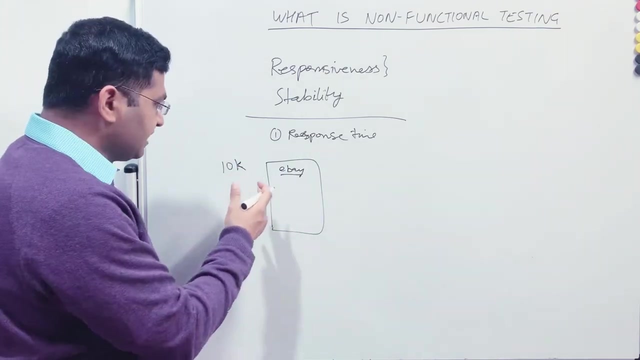 time time. so, based on, say, for example, 10 000 users are concurrent users- are accessing ebay website at one particular time, how is the response time for the user that is trying to access at that particular peak time right? so whether the website is loading within five seconds. 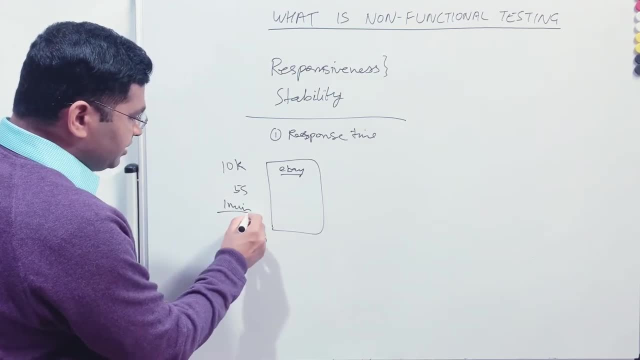 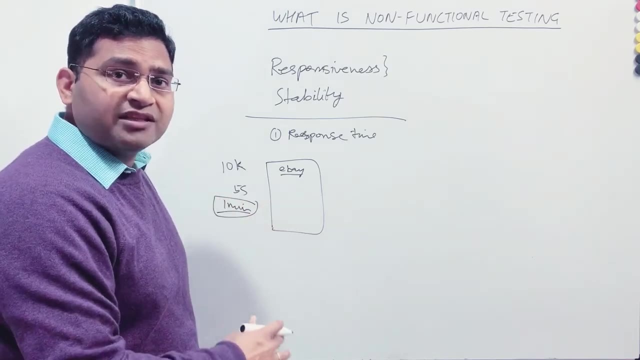 or it is taking, you know, one minute, okay, so if this is not acceptable, if this is, you know, taking a lot of time, then you are verifying the response time and then you are verifying the response time, right? so if there is a lot of time, there will be a lot of users frustrated and they 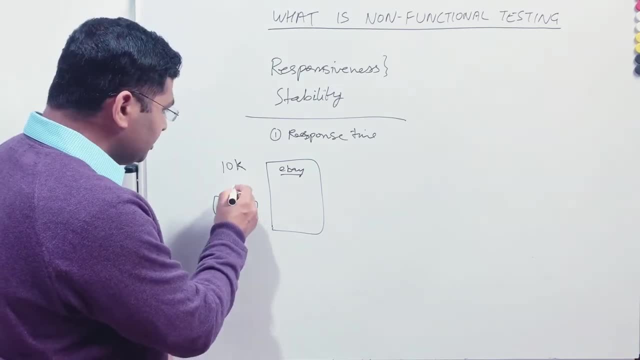 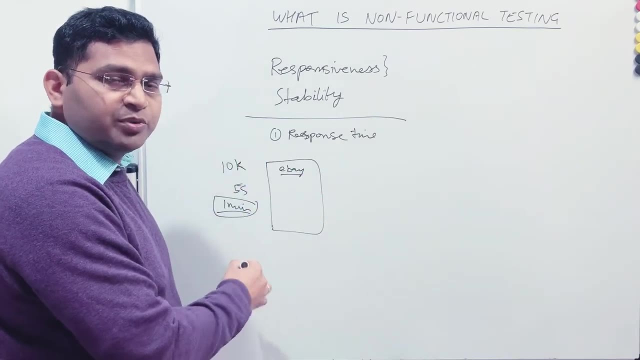 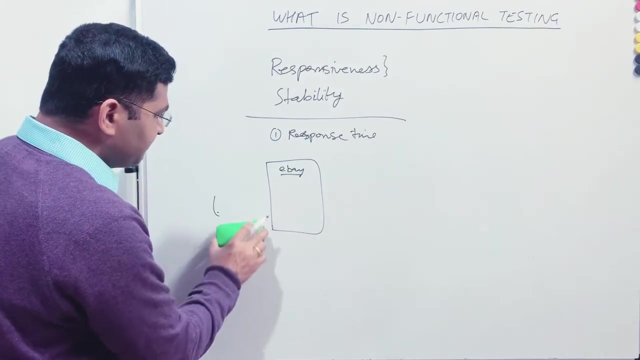 leave the site and they won't access it, right? so this is what, basically, the response time is all about. so when you know, during a peak load of time, peak load- what is the response time and normally what is the response time. so if you are verifying the response time, so that is one of the factor. 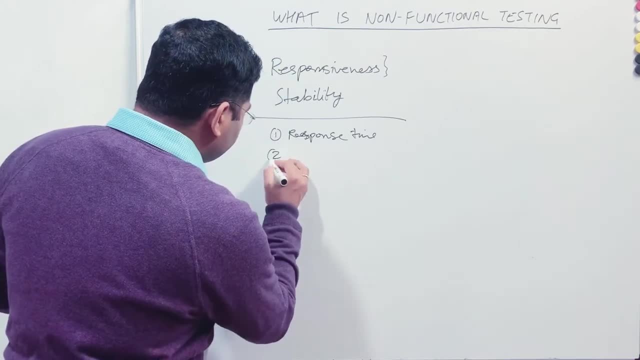 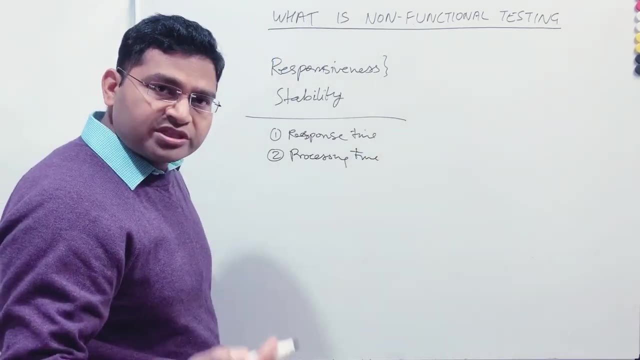 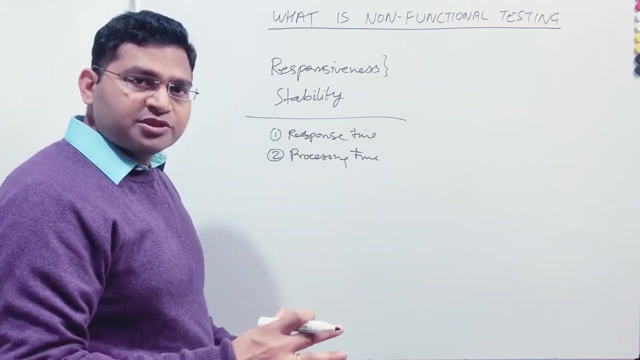 in non-functional testing or the performance indicator. the second one is the processing time. right, so processing time. so when we say processing time, how much time it takes to process? say, for example, a customer came to the website and they added the order. they added items in the order and submitted order, made the payment. so, after making the 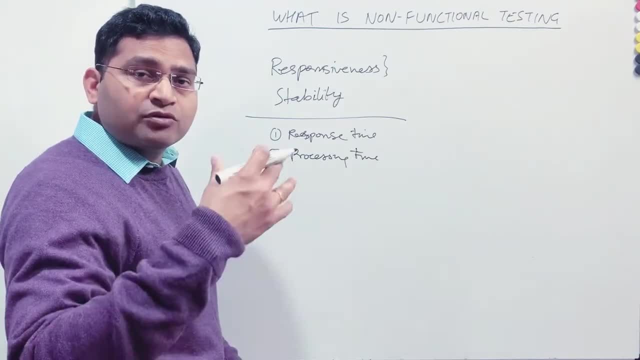 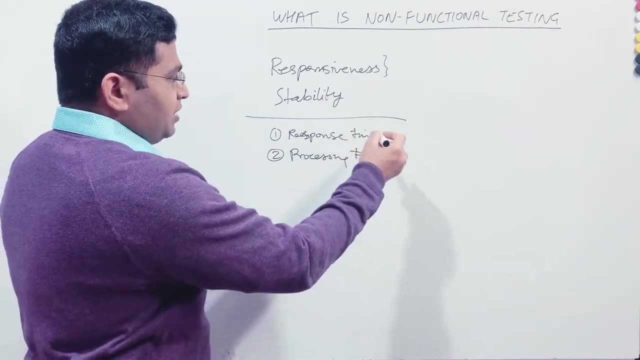 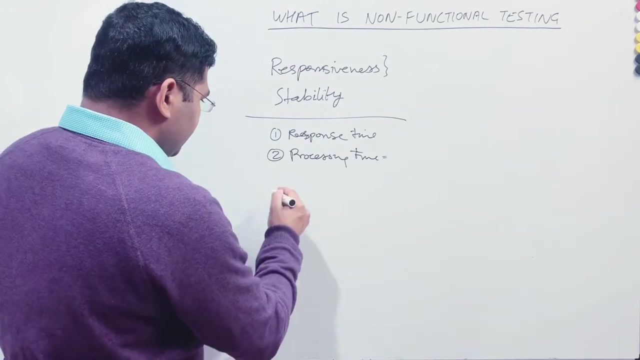 payment, how much time it took to process that whole payment and send the response back to the customer. so that is the process time, or processing time. so this is one of the second indicator that you mostly check into, the non-functional testing or the performance testing. the third one is the concurrent user volume. 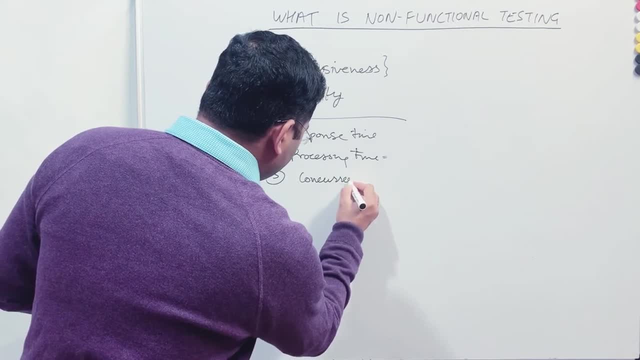 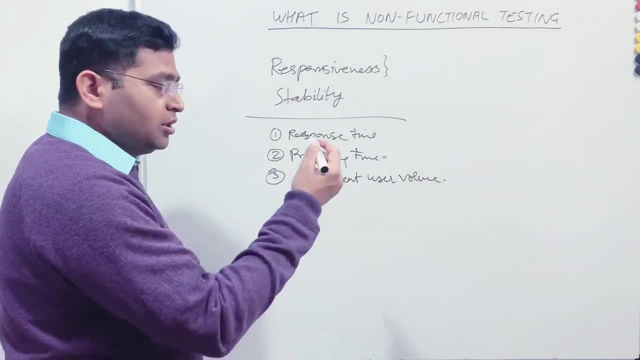 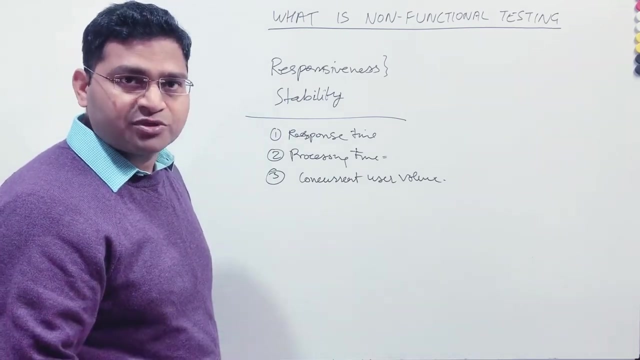 right. so concurrent user volume: okay, so concurrent user volume, we have already touched base on it. so say, for example, there is a sale going on, there will be thousands and thousands of content user trying to buy the on sale items on the e-commerce website. so you verify the. 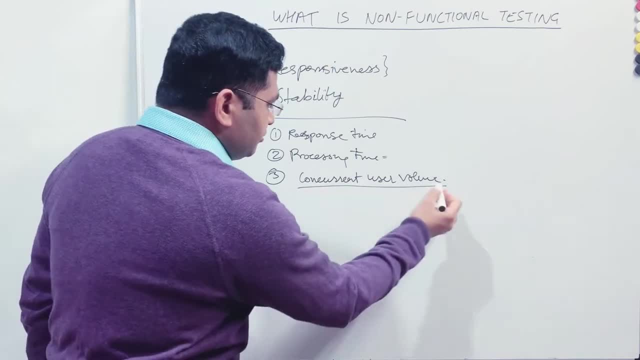 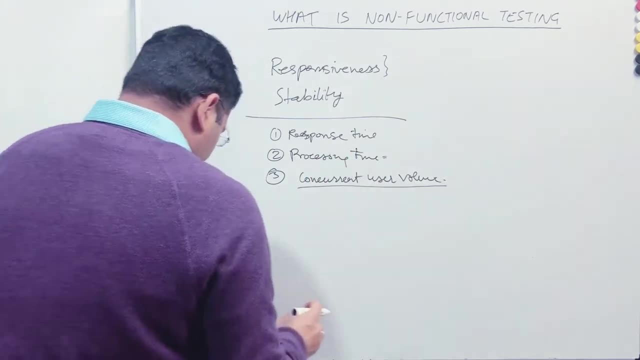 you verify the on sale items on the e-commerce website so you verify the responsiveness and stability of the application during you know concurrent user volume or when there are lots and lots of user at one particular time. so these are some of the performance indicator and, in the non-functional, 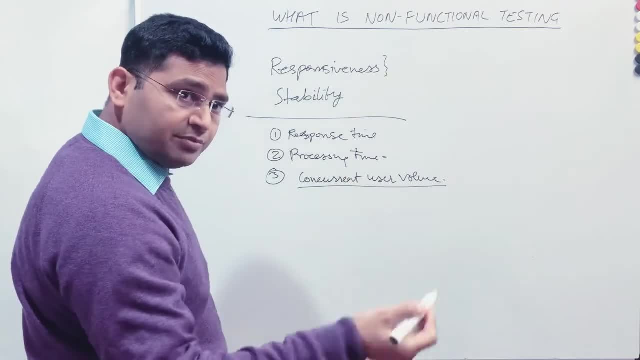 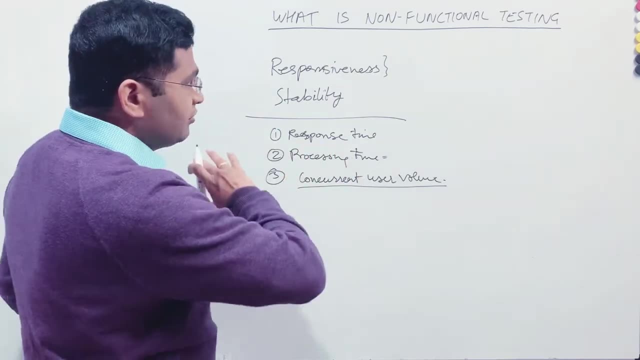 testing or performance testing, you basically verify how reliable your application is, how robust it is. so all these are some of the factors you consider in the non-functional testing. now let me cover what our main type of non-functional testing or performance testing is and what are the main types of non-functional testing or performance testing. 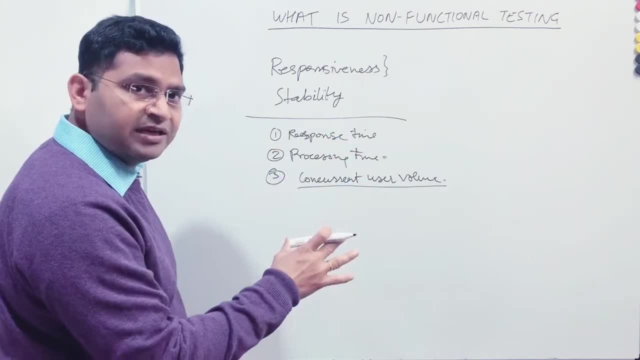 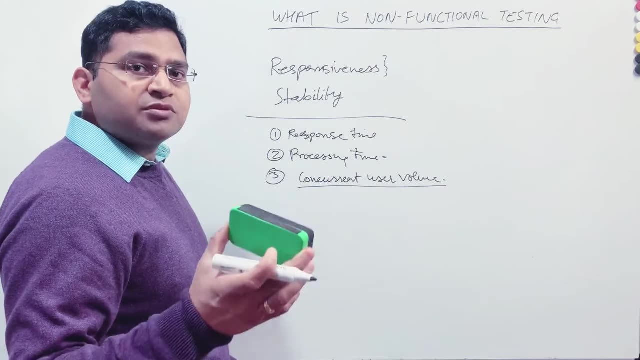 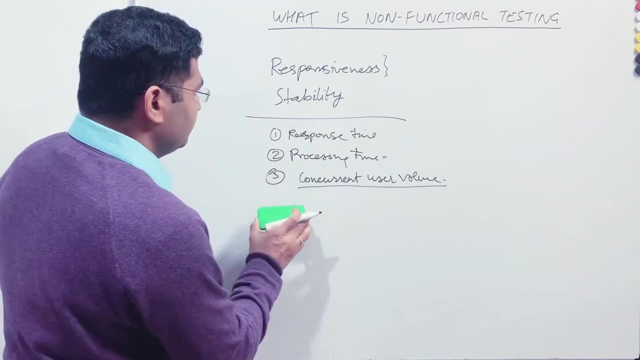 that we do so. performance testing is one type of non-functional testing and within performance testing there are many subtypes, right? so the main subtypes will cover in this particular tutorial and then I'll also cover those subtypes with example in upcoming tutorial, right? so let me remove this and the first. 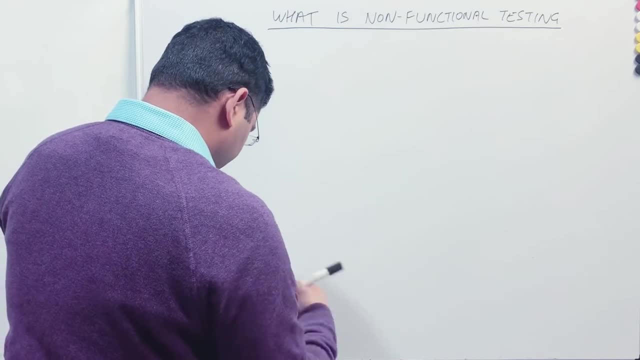 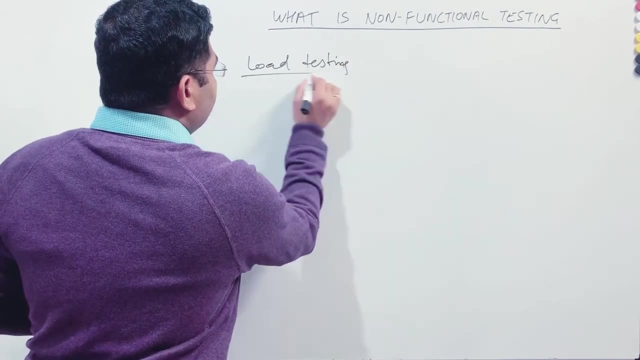 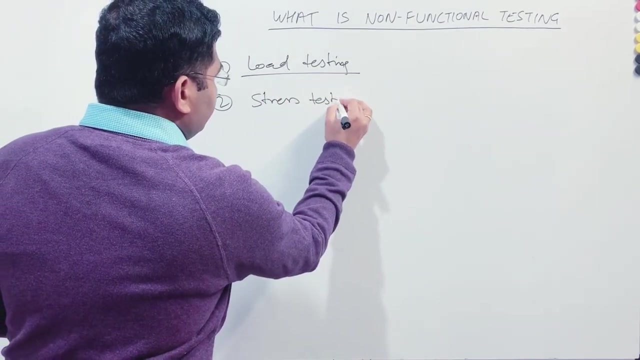 non-functional testing or, you know, the performance testing I want to cover is load testing, right? so load testing, this is very common, you would have heard, so let me write all of those. so load and then stress testing. so these are the common types of non-functional testing or the performance testing that you will. 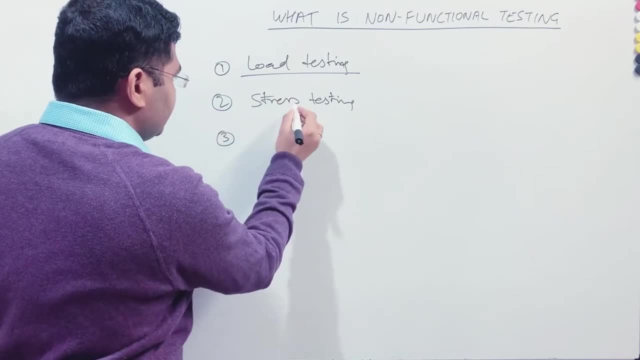 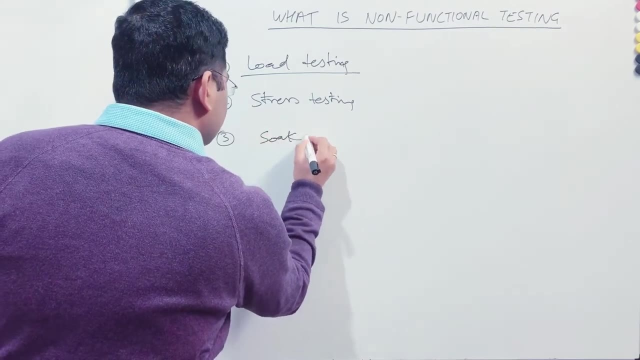 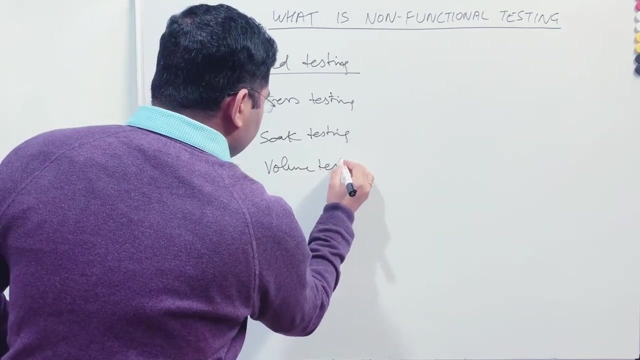 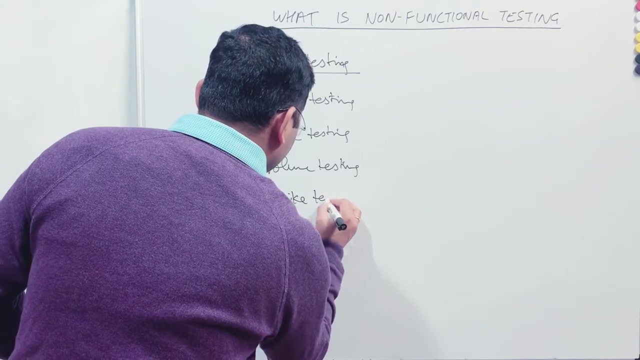 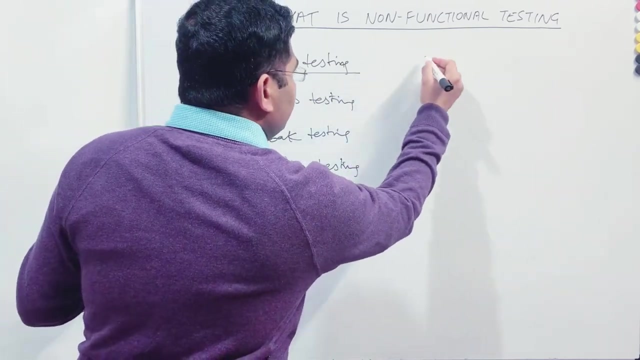 hear, and you need to understand all these in detail, right, so that you can explain to the interview. the third one is soak testing. so soak testing. fourth one that will explain is volume testing and fifth one is spike testing. okay, now let's start with load testing. so say, for example, you have the e-commerce website. 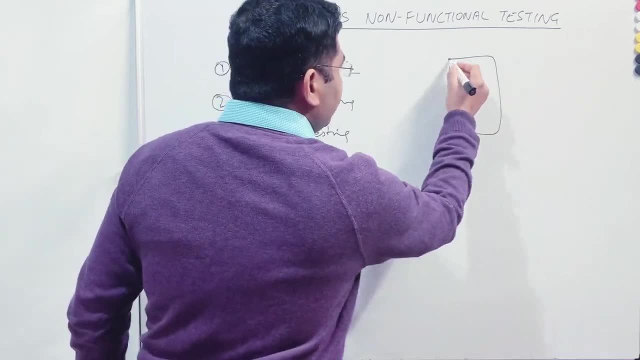 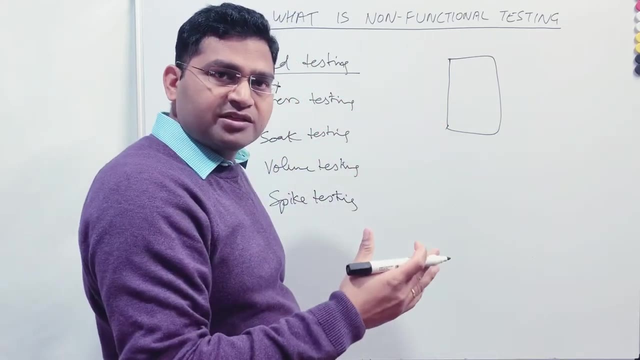 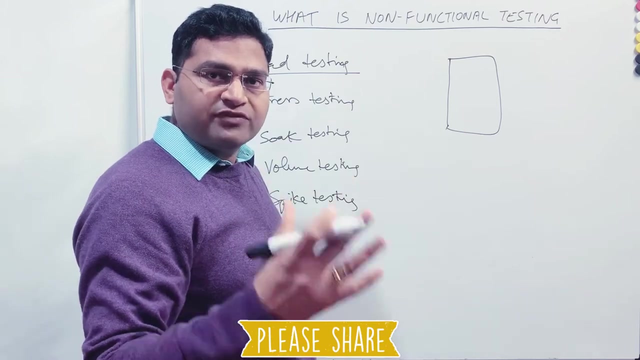 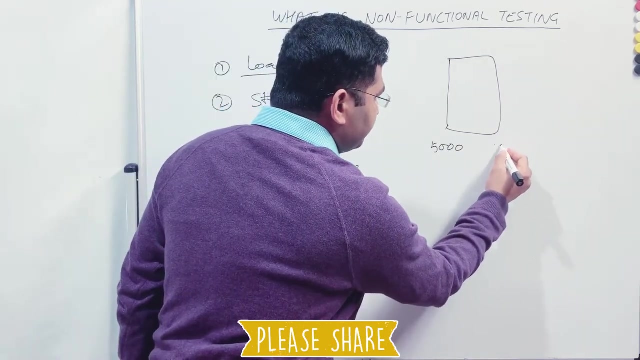 okay, and in this particular application, your customer has given you the non-functional requirement. say: I want this particular application to work perfectly fine, up to 5,000 concurrent users, right, so up to 5,000 concurrent users. the response time for this particular website should be less than you know five seconds. ok, so in this particular 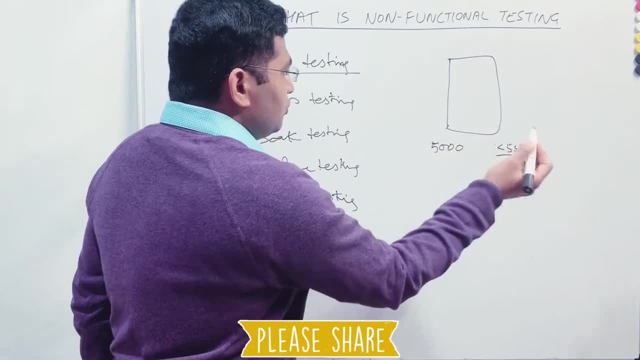 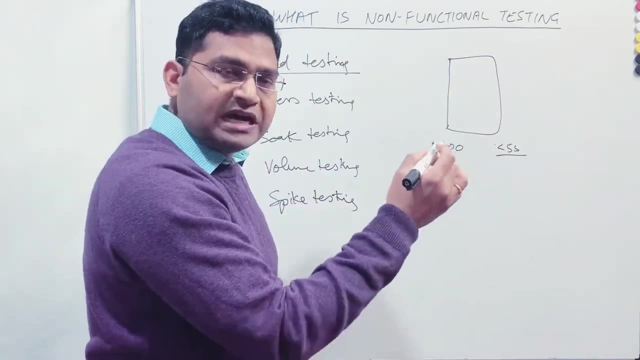 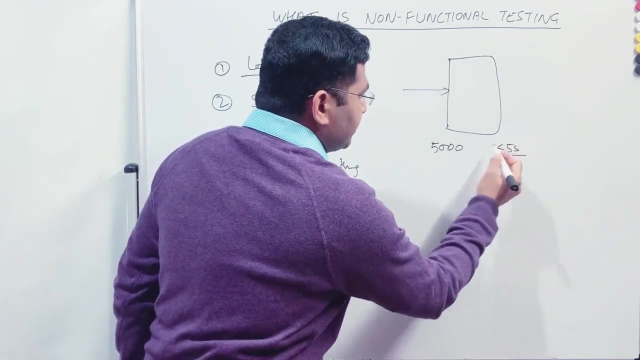 case, what you do in load testing is basically you verify that when the 5000 concurrent users are accessing this particular application, the response time that you are getting should be less than five seconds. so when there are 5000 concurrent users accessing the particular website. so in the manual, 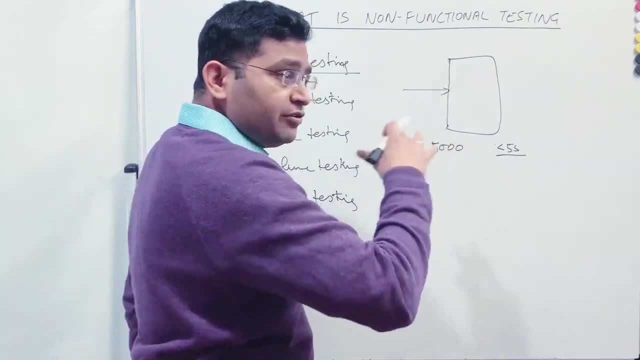 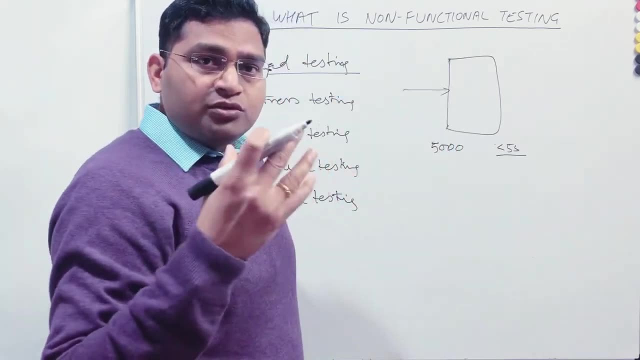 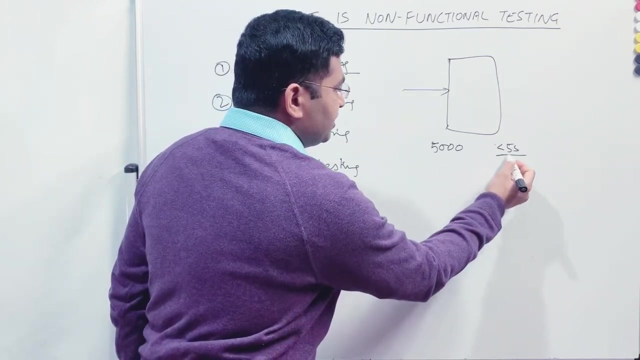 scenario what you can think of is say, for example, you 5000 people accessing ebaycom right or any application they are trying to build, and when you are the 5000 user and for you the response time should not be more than five seconds. but in the actual scenario, in the real testing, it is not. 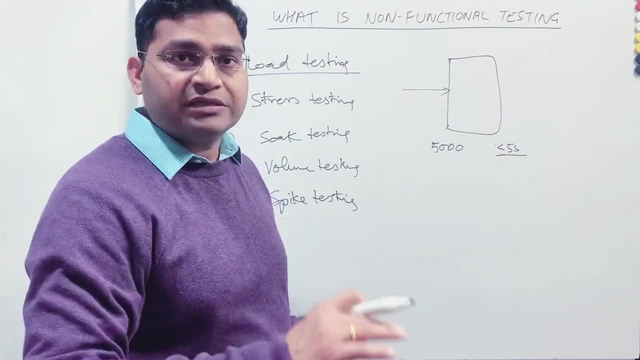 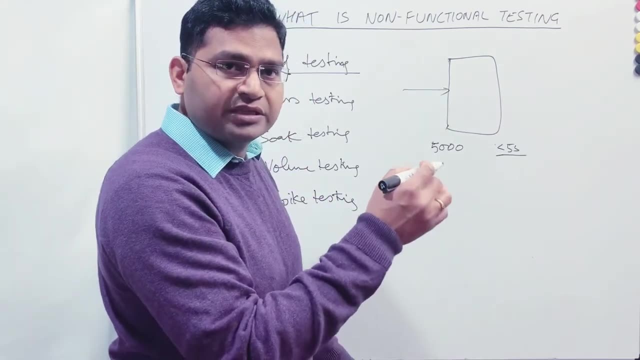 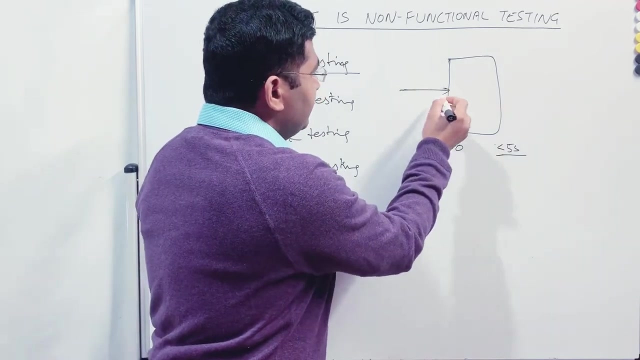 possible to have the 5000 concurrent physical user trying to hit the server. it is only possible in the production. so, in the testing scenarios, what is done is the usage of tool is there. so with the tool, the 5000 concurrent threads are being, you know, created and this, you know, simulates the users, 5000 users, and the response time is. 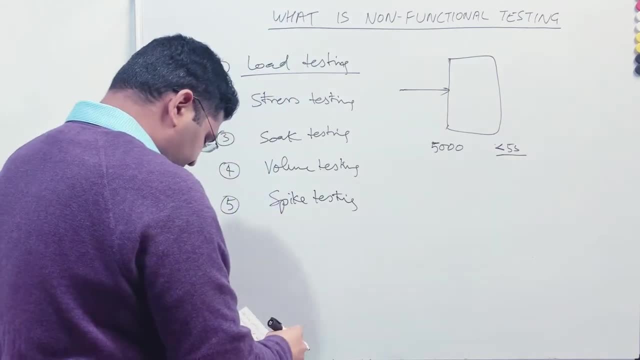 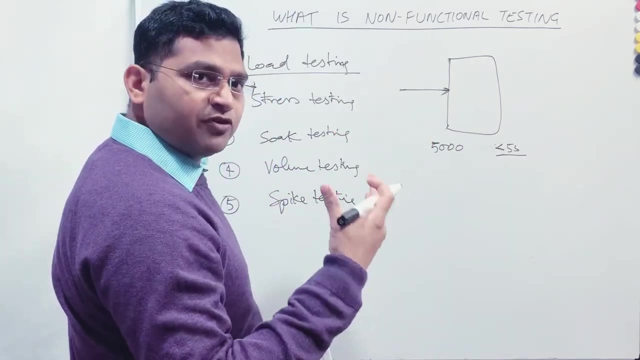 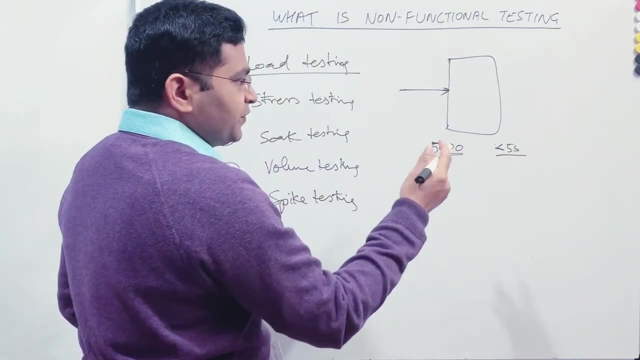 checked whether it is less than five seconds, right. so this is what your load test is all about. so testing the performance of the application on a particular load that is given by the user. so if your application is performing or the response time is within the accepted limit as 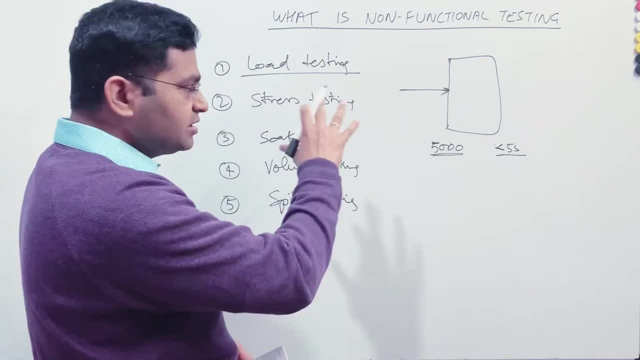 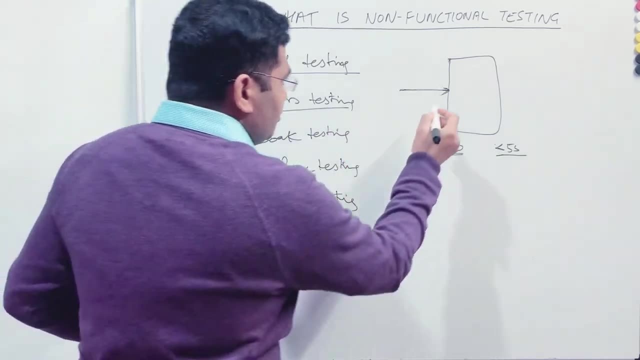 provided by the user, then you can test the performance of the application on a particular load by the customer. then your load testing is fine. so this is what load testing is now when we talk about the stress test. okay, so now load test is verifying that the response time is within the 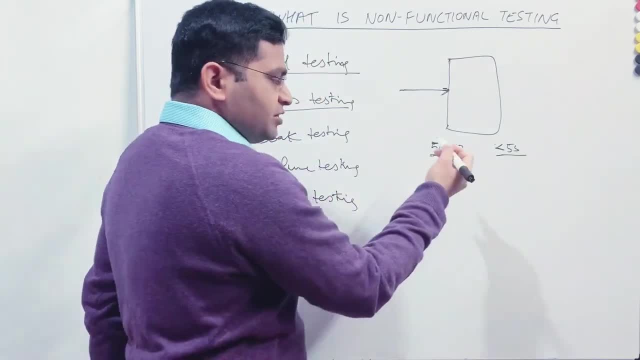 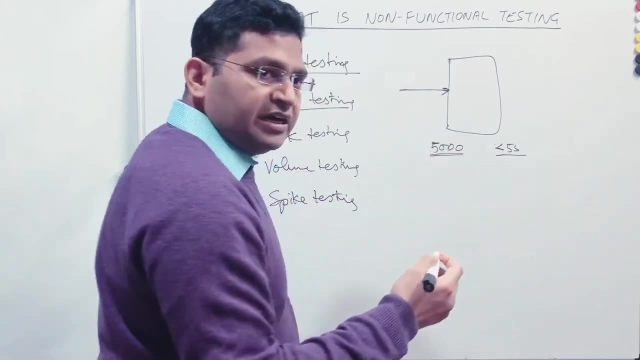 expected limit when there are 5000. so, for example, concurrent users, which is the requirement from the customer. in terms of stress testing, what we do is we verify the, we stress the system or we increase the stress of the system and we increase the stress of the system and we increase. 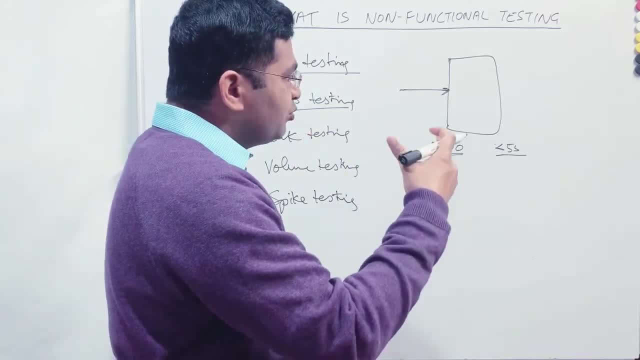 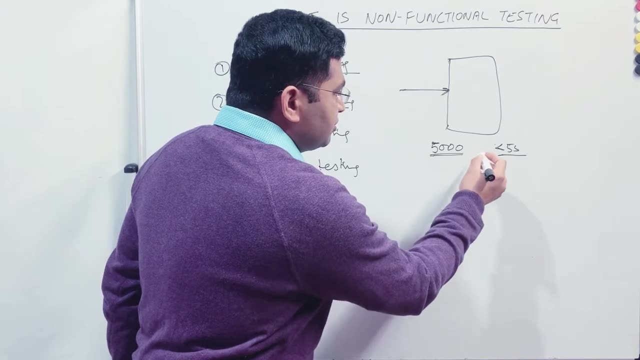 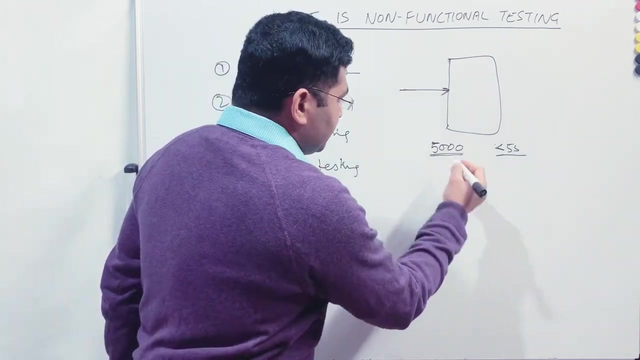 the number of users and verify at which particular point of time the application will break. okay, so, for example, the requirement is 5000 users and the response time should be less than five seconds. now, this is what you will verify in load test, but in the stress test, what you will do is you will. 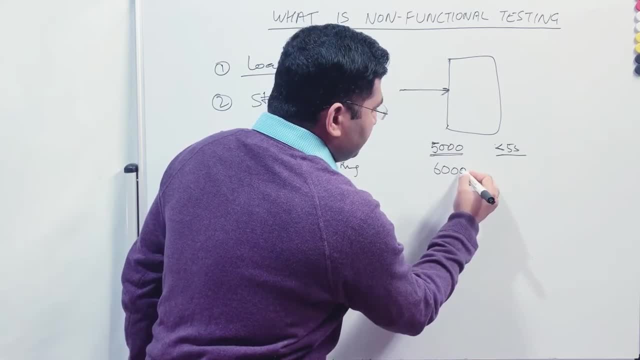 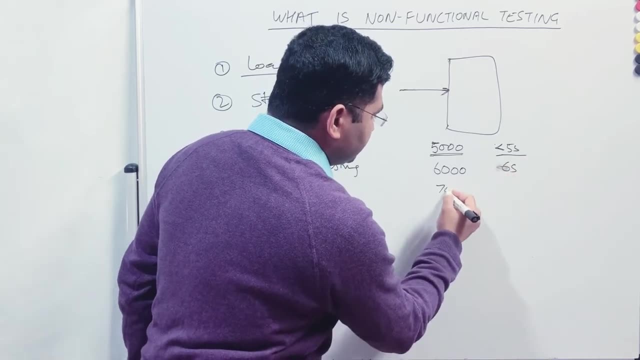 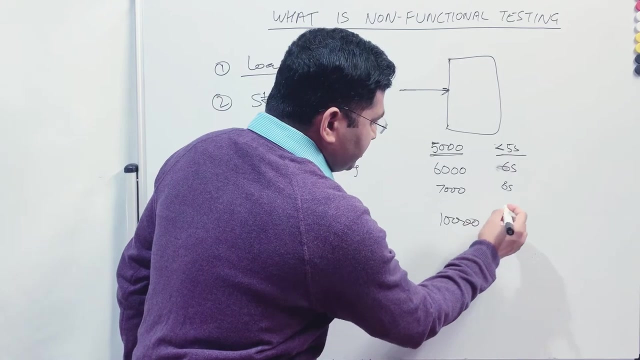 increase the users to 6000 users and then say, for example, once you increase it to 6000 users, the response time was, say six seconds. right, then you will increase it to 6000 users, and then you will increase it to 7000. response was eight seconds. so you will keep doing it until the application. 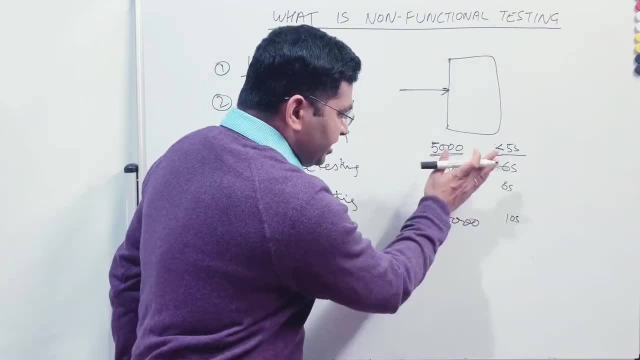 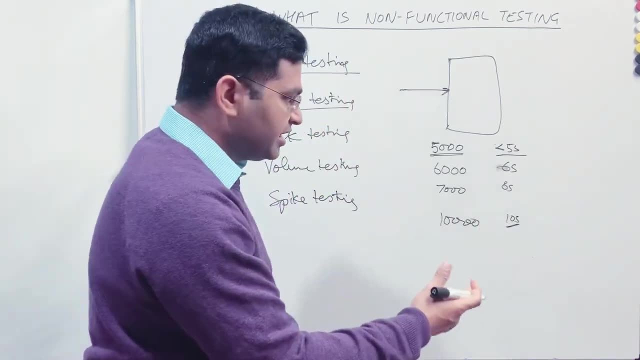 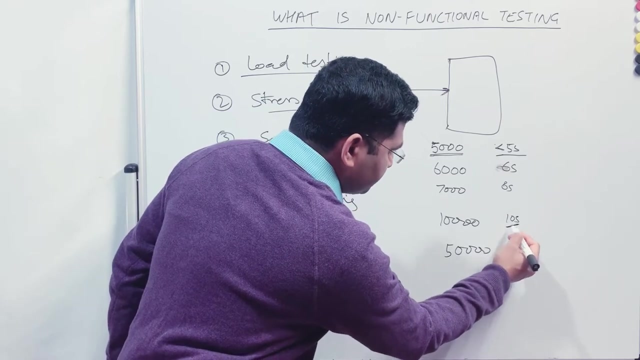 breaks, okay. so you, you just keep making note of what is the response time and what is the point when the application crashes, crashes, okay. so, for example, here you have now increased to you know, 50 000 users, concurrent users trying to access the particular website, and the response time is: 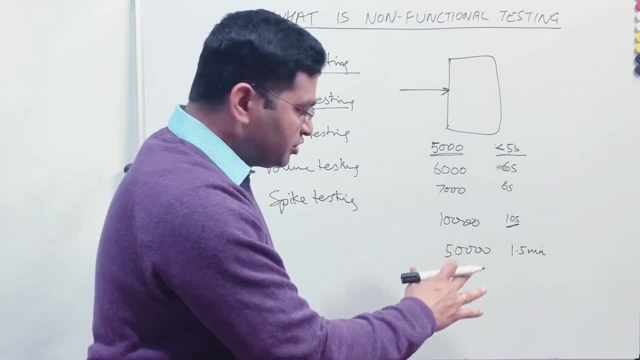 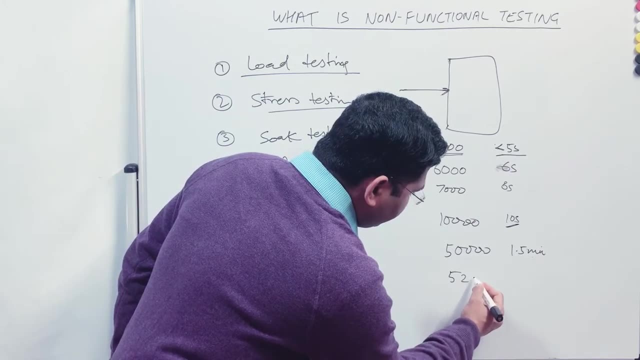 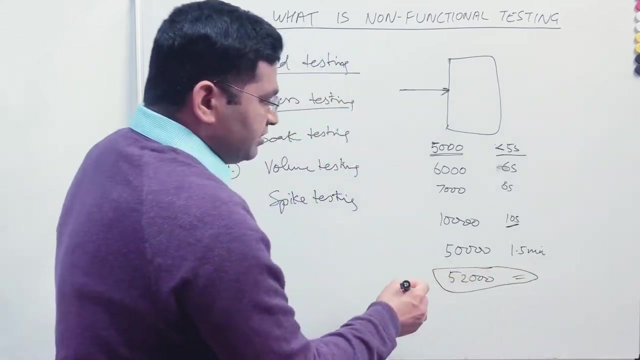 five minutes, okay, so this is very high response time, but you keep increasing the load, okay. so you keep increasing the user and say, for example, at 552 000 users, um, you know, the website crashed. so this is the point. that is basically the crashing point, and this is what you do in the stress testing. 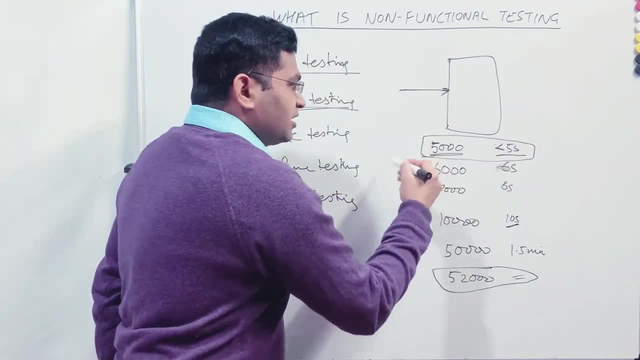 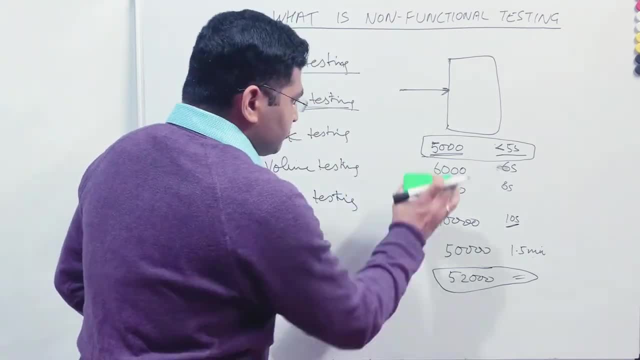 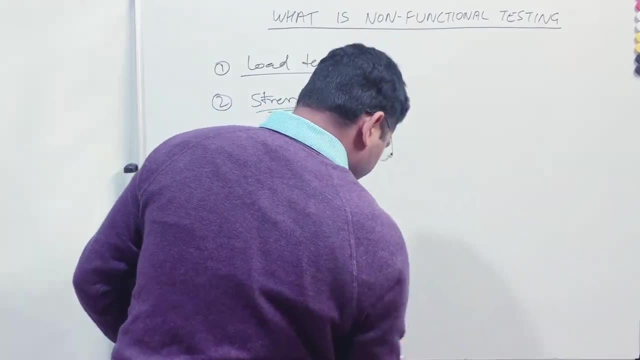 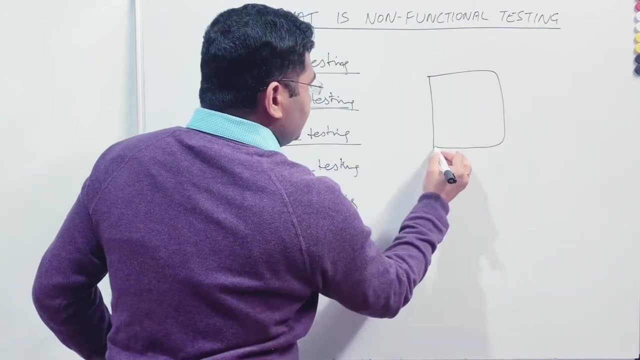 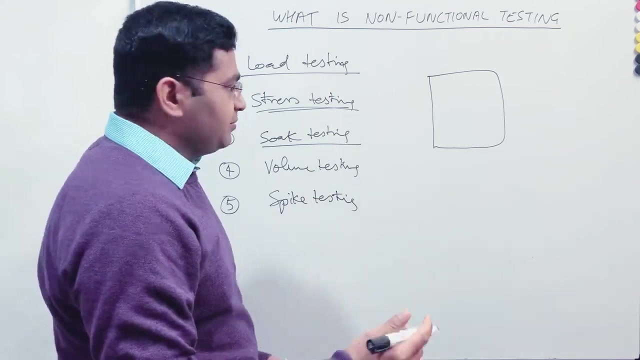 the load, so you keep increasing the load, so you keep increasing the load, so you keep increasing. So this is what you do in the stress test. Now coming back to the SOAP test. So in the SOAP test what you do is so as we have done in the load test. in the SOAP test you run the load test up to in the longer duration or up to extended period of time. 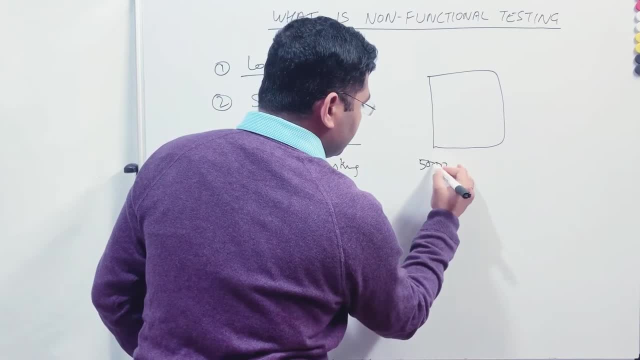 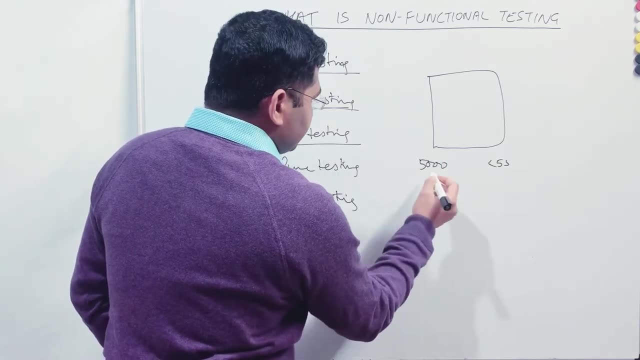 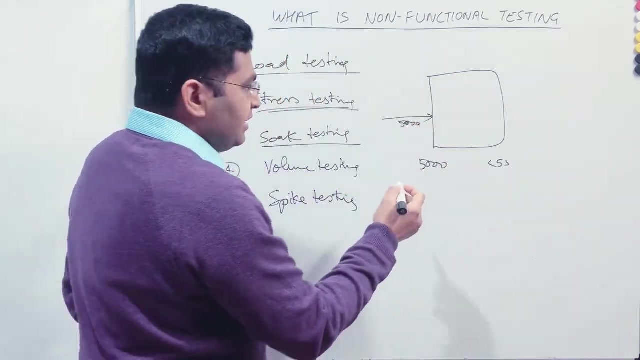 Right. So, for example, the requirement was 5000 users. concurrent users. Response time should be less than five seconds. OK, now what you do is SOAP. test is basically you create 5000 concurrent users accessing that particular website and that test runs for a couple of hours or a couple of days, based on requirement. 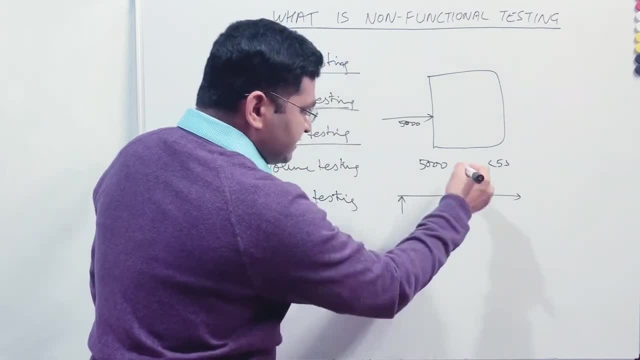 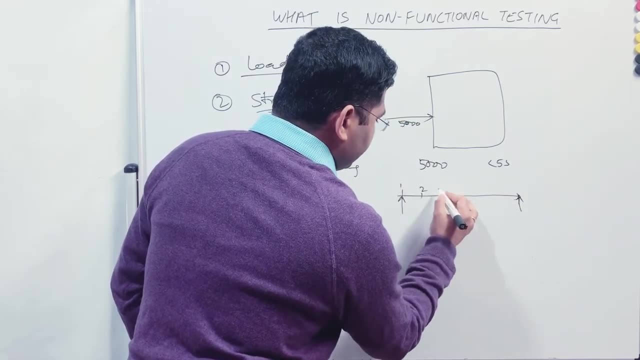 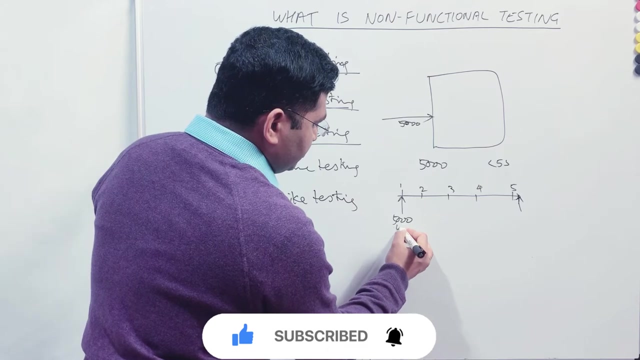 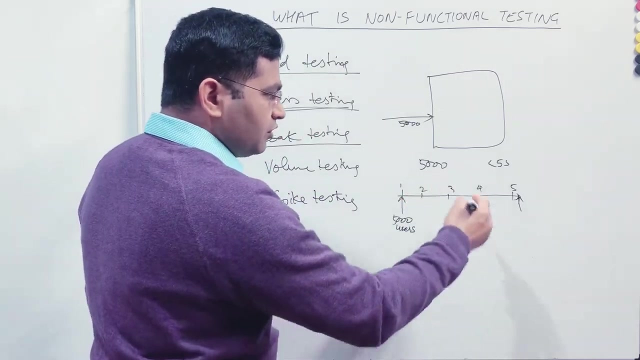 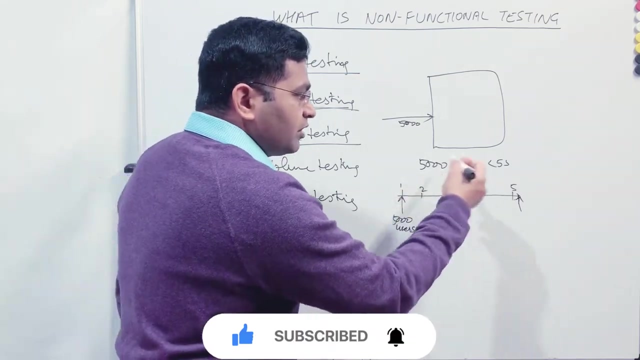 OK. so say, for example: this test needs to run for five days. OK, So first day and then second, third, fourth and fifth, OK, so you create the load here of 5000 users, OK, and then that load continues for five days and you test that the different operations with that load for up to five days. 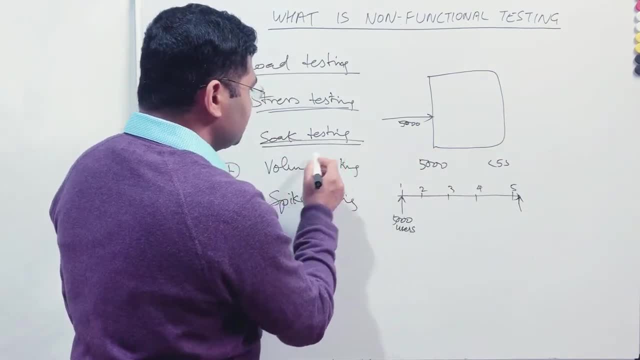 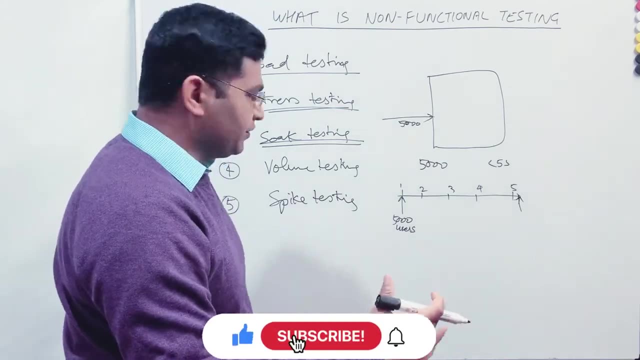 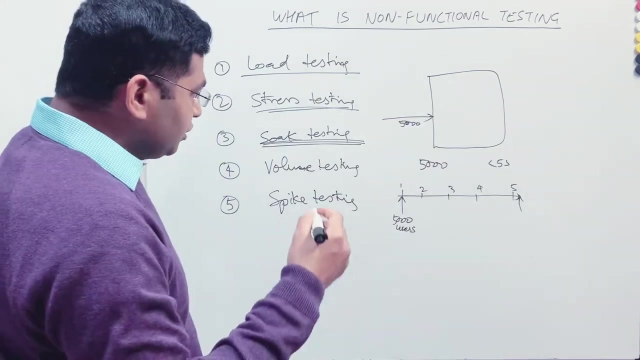 When you do that type of testing. it is known as SOAP testing. So basically, you are, You know, running the test for extended period of time on the peak load. OK, so that is what SOAP testing is all about. Then, if we talk about the volume testing, you know volume testing is mostly it's relevant for the testing of the database of the application. 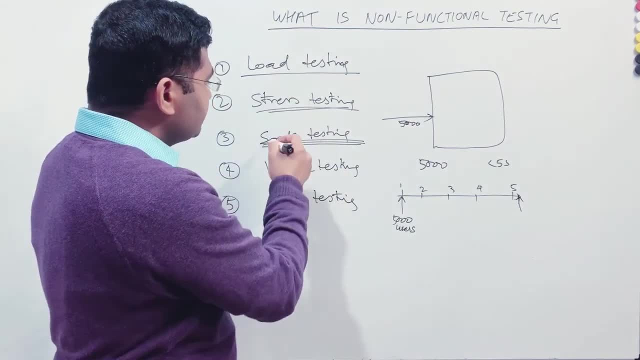 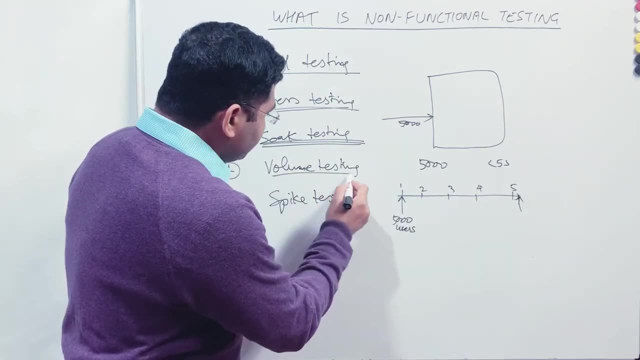 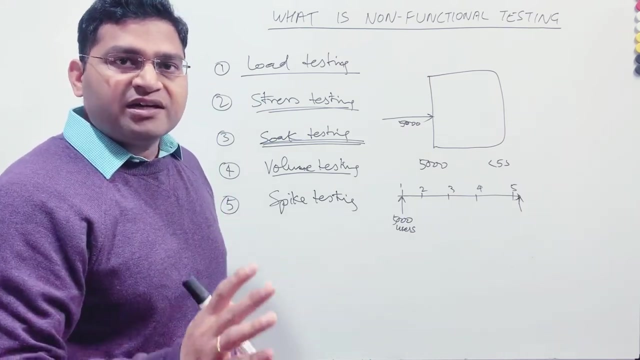 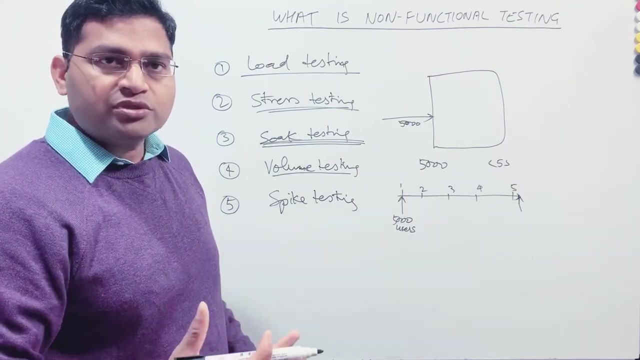 Right. So here we are more concerned: load stress and SOAP. We are concerned about the users, concurrent users accessing the website or the portal. But when we talk about the volume testing, It is about the size of the database. or when you input a lot of data into the database or you fill the data completely or reduce the size of the database. 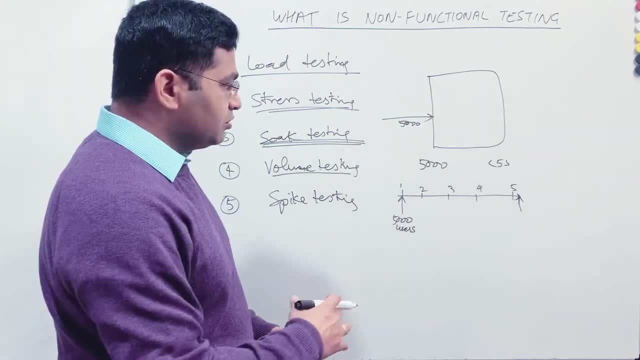 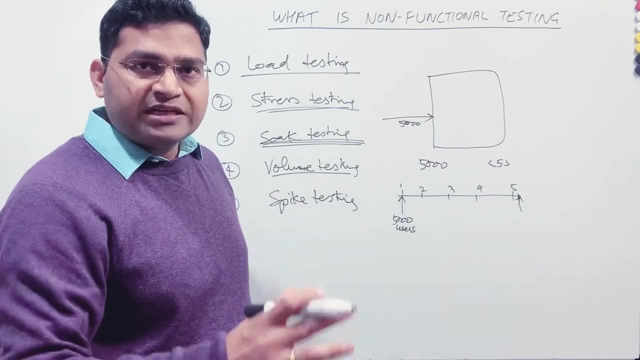 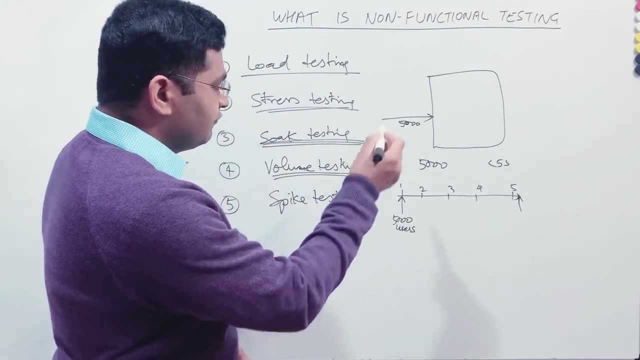 Right, Not not reducing the size. basically Say, for example, your database size is of five GB and for that five GB database you fill it up and then verify how the application behaves. Then that particular you know type of testing or the non-function testing is known as volume testing. 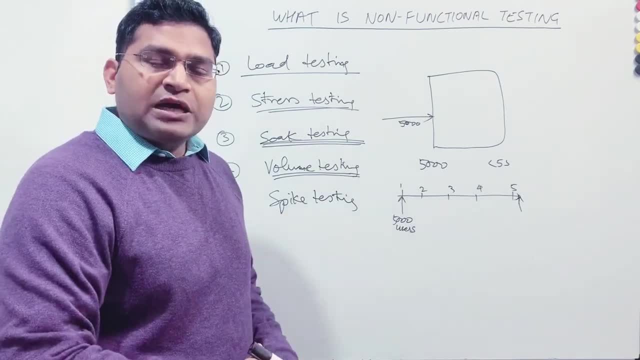 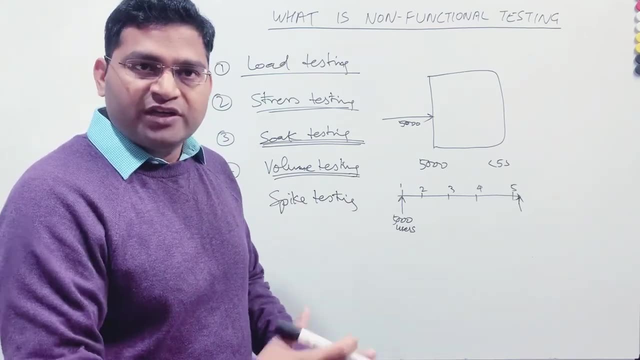 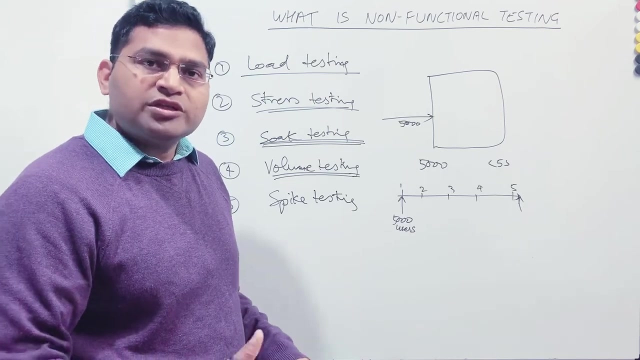 So this is important because, say, for example, you have the e-commerce website and when you start getting lots and lots of order, your database, or database, will fill Right. So once your database is full or near full, how the application behaves, or what is the point when the when the application will crash. 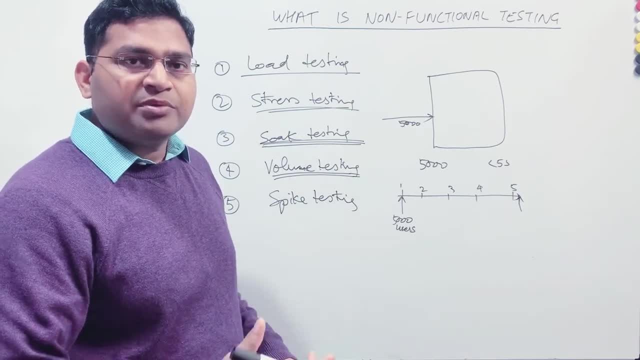 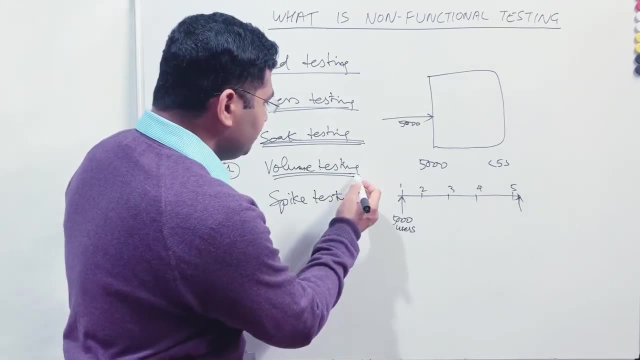 So that sort of testing is also important. Say, for example, the, The space is not left, the database is full. then how the application will behave Right. So that is the volume testing. Now spike testing is another type of testing, non-functional testing. 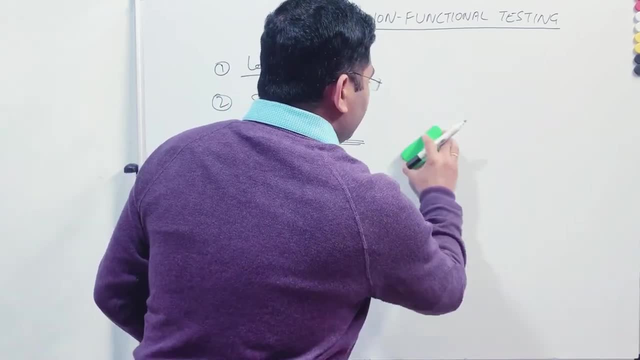 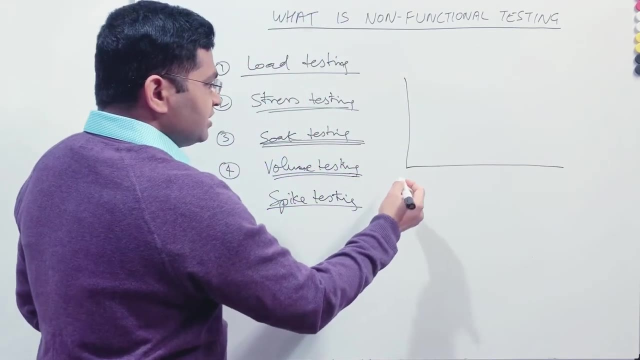 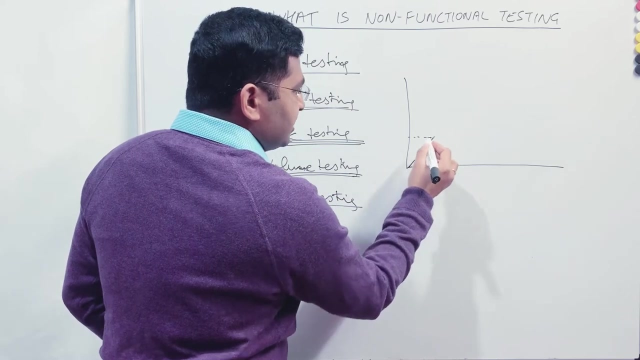 What you do in the spike testing is in the load testing we have the load of 5000 users. So basically, how we create the load test is so there is a ramp up and then, as soon as so, in the ramp up phase, the number of users are the threads. 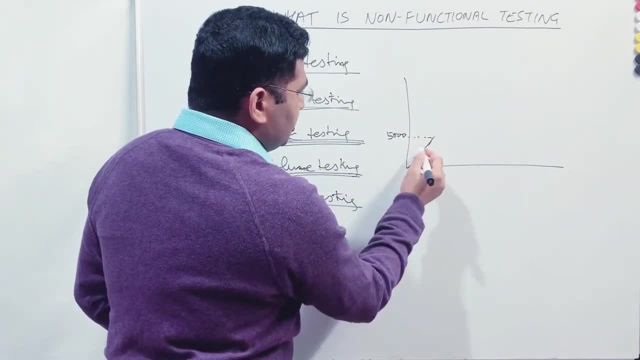 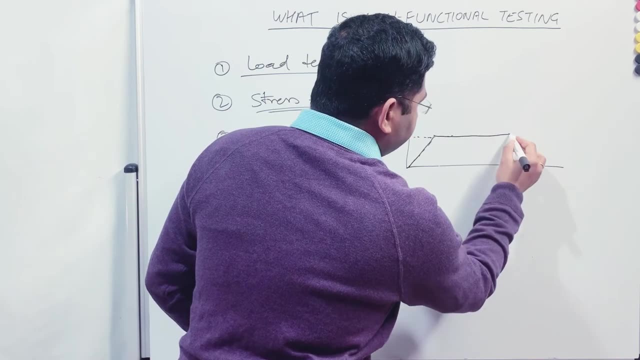 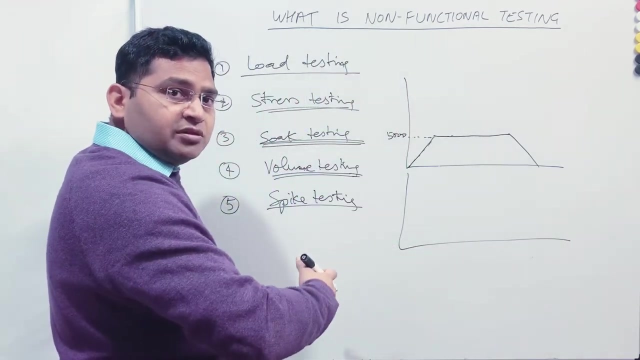 Increased and up to 5000 users with the tool. and then you know you have this 5000 users. you do the test and then you ramp down. Right now in the spike test what happens is there are sudden spikes of users and then sudden- you know- reduction of the users. 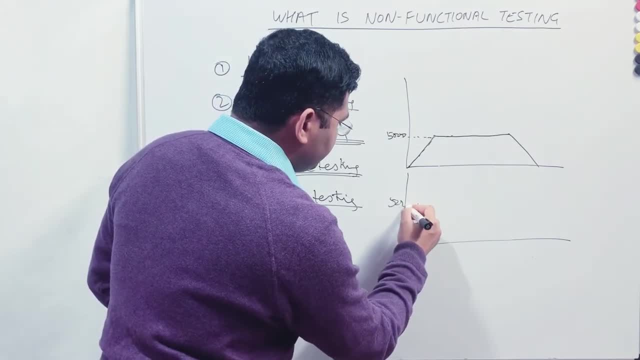 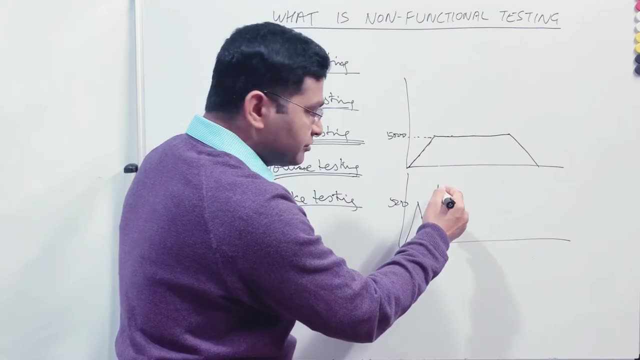 So what happens is suddenly there will be like 5000 users and then there will be, you know, like no user, or reduced to the half, and then sudden increase To the user to the 10000, and then reduction to zero, and again. 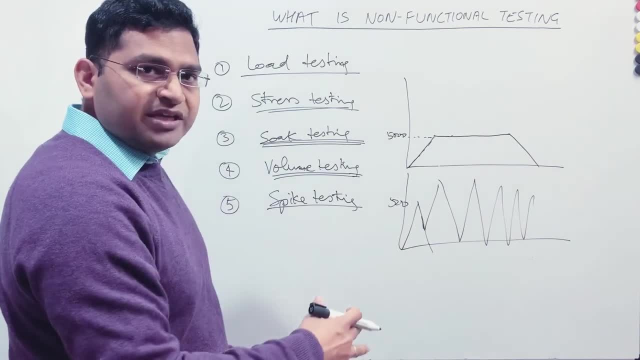 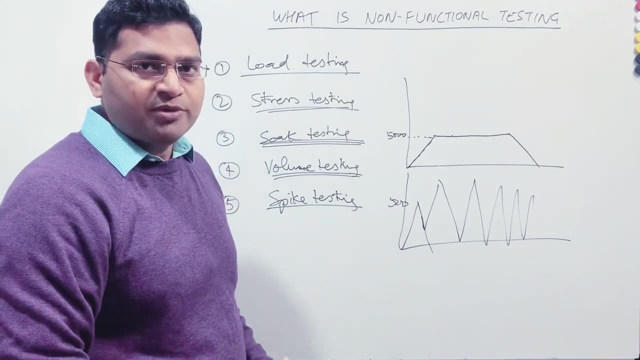 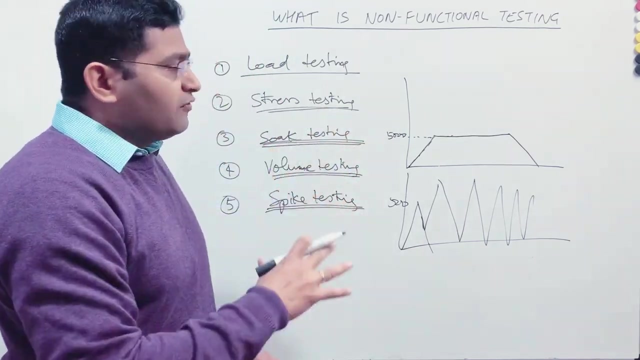 So there is a spike of users on the application and then reduction of the users from the application and then verify how the application is performing in that particular scenario. So that is known as by testing. So these are some of the non-functional testing. There are many more non-functional aspects and non-functional testing. 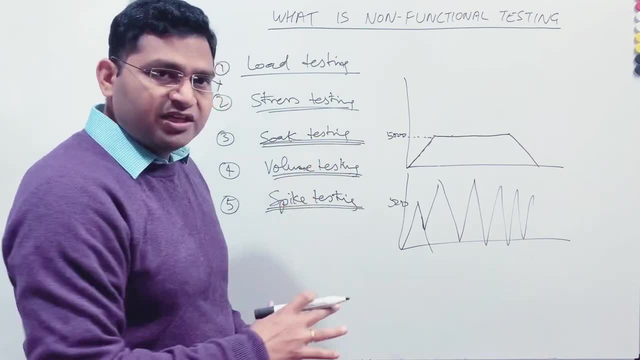 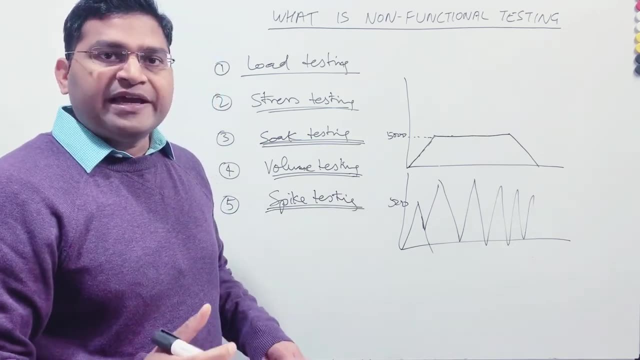 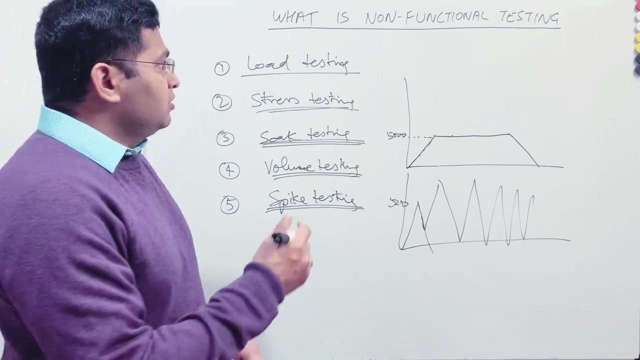 But in terms of interview, these are the five key. You know non-functional testing. that should be good enough for you to explain what exactly non-functional testing is and why non-functional testing is required in any application. So non-functional testing is required to you know. verify the reliability, how robust the application is. 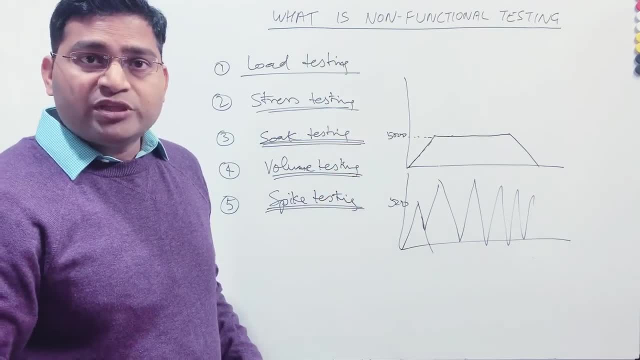 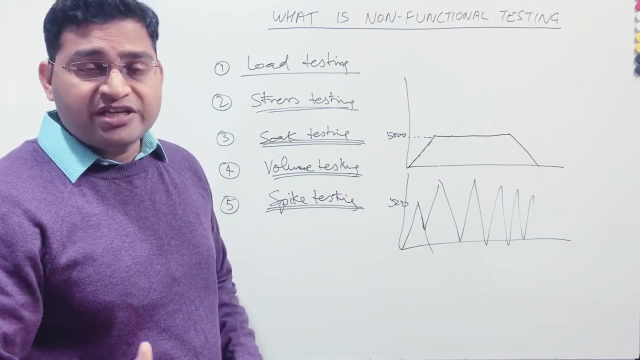 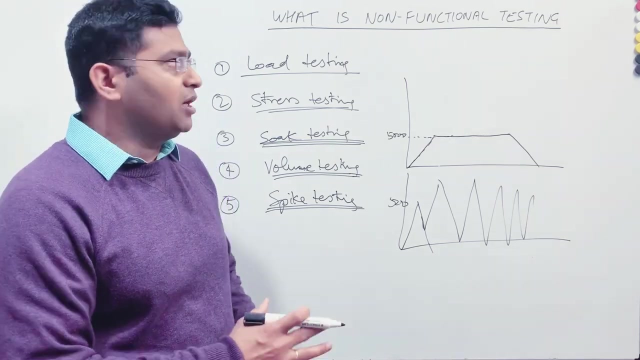 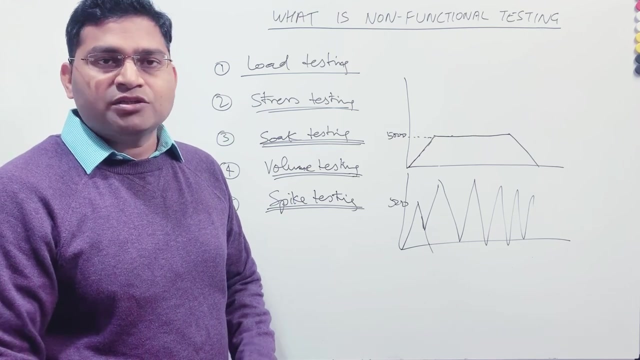 Right. So, as we have seen, basically what will be the response time, whether whether the application is available on the high load or high volume, or if the database is full or near full. So these are some of the Scenarios that you can explain in your interview when somebody asks you about what is non-functional testing and what are types of non-functional testing that are commonly used and you will hear very commonly in your projects. 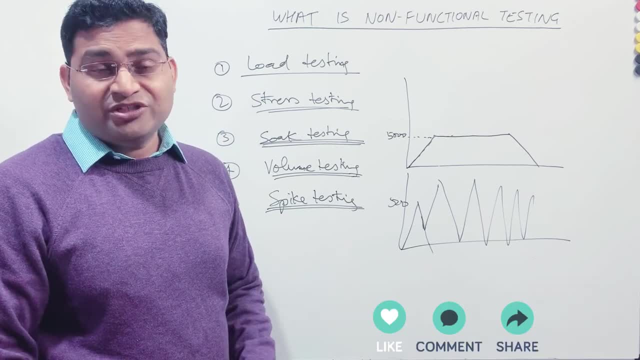 OK, so that's all for this tutorial. Hope it was helpful. Please do share and subscribe, And thank you very much for watching.